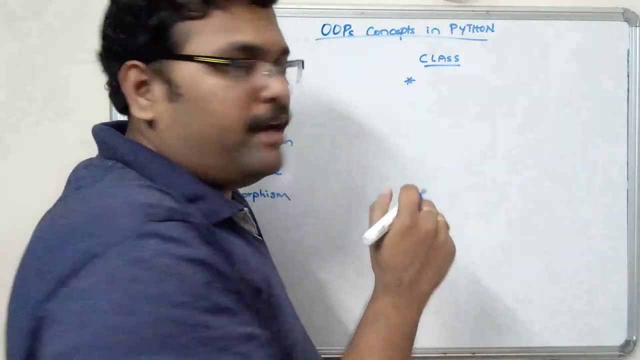 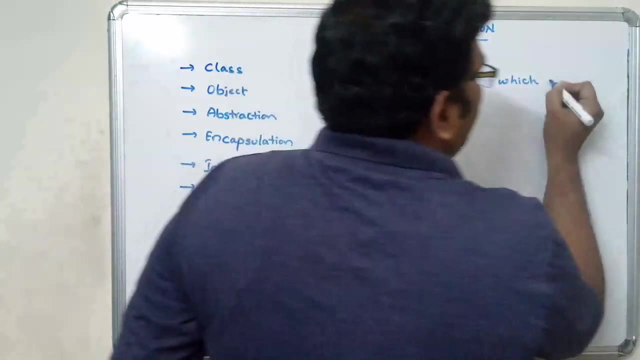 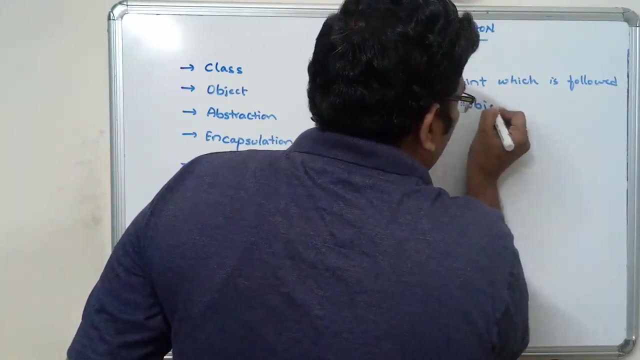 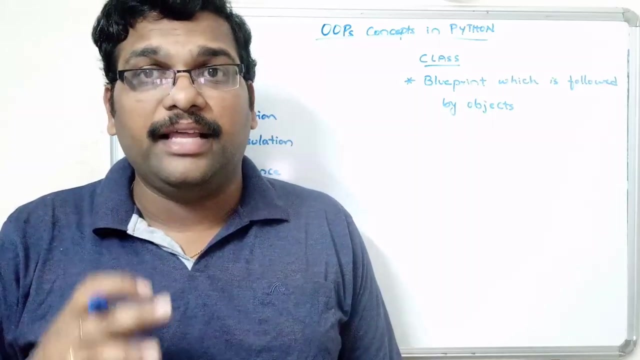 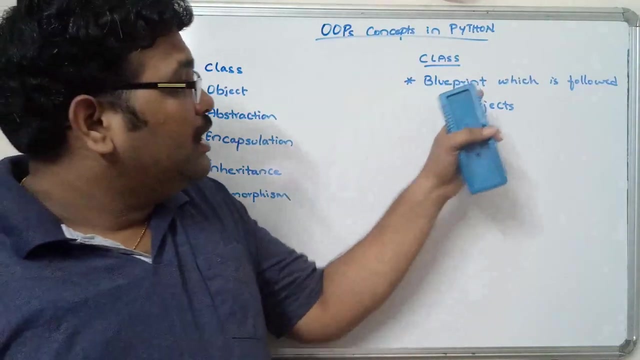 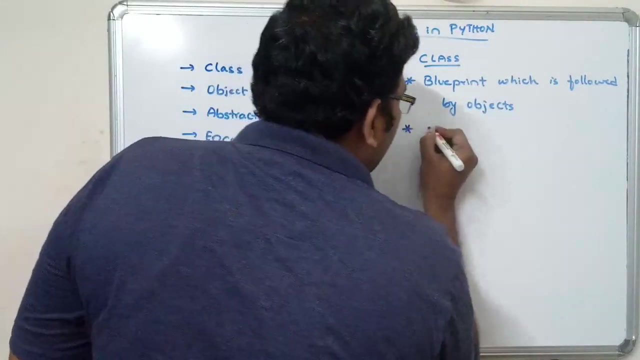 Okay answerớ. so it is a blueprint which is followed by objects. so here every class can have a multiple instances. so here the instance means object. so every class can have a multiple objects. right, so that object should follow the blueprint of the particular class. so that means it is a logical structure, the class can be. 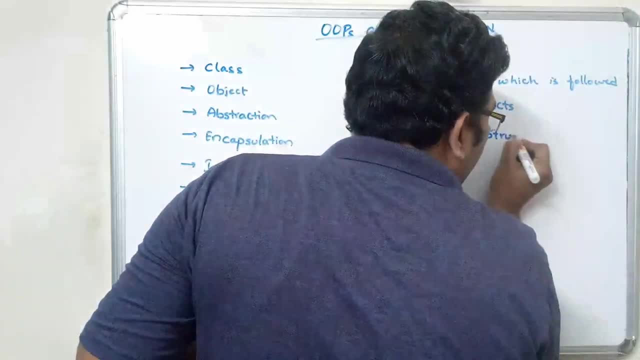 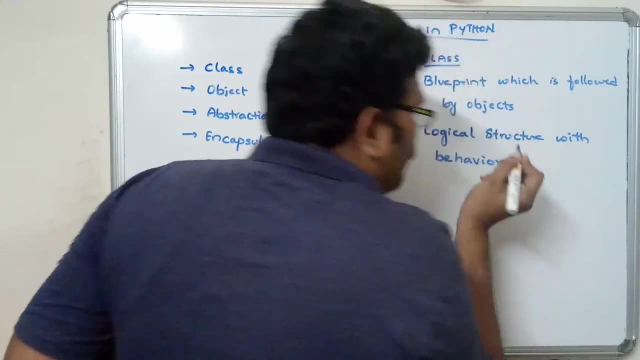 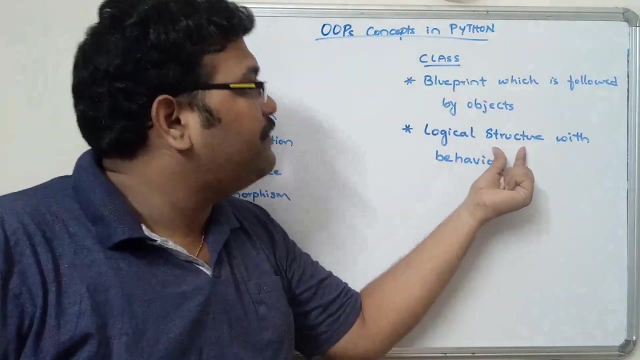 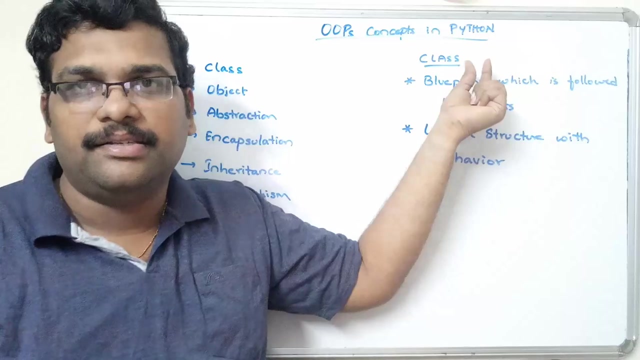 defined as a logical structure with the behavior, with the behavior right. so whatever the blueprint or whatever the class is, it should be a logical structure, the structure we define for the class, that should be followed by the objects which are created for that particular class. so these are called instance of a. 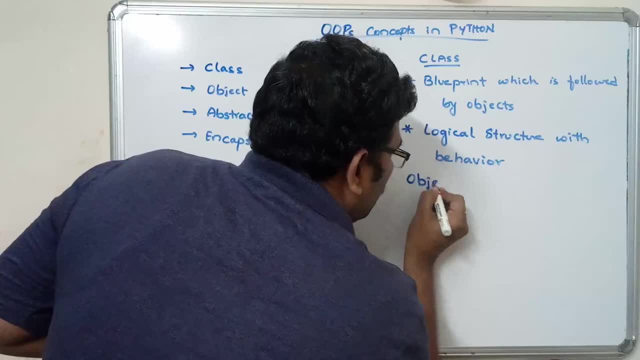 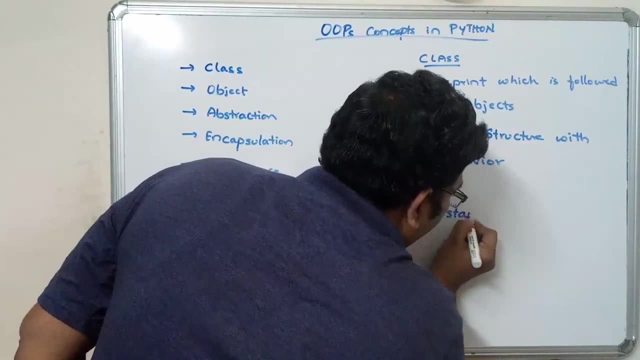 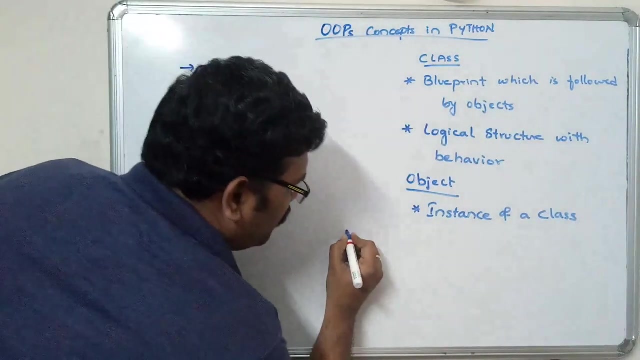 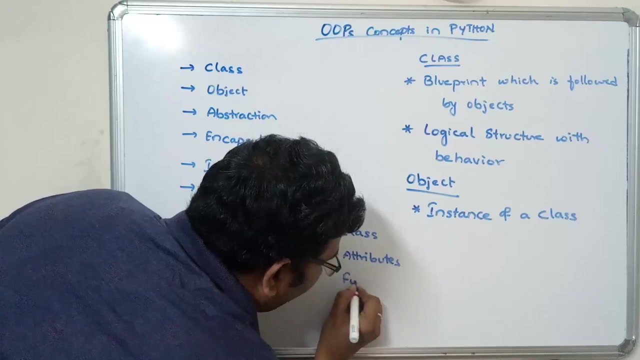 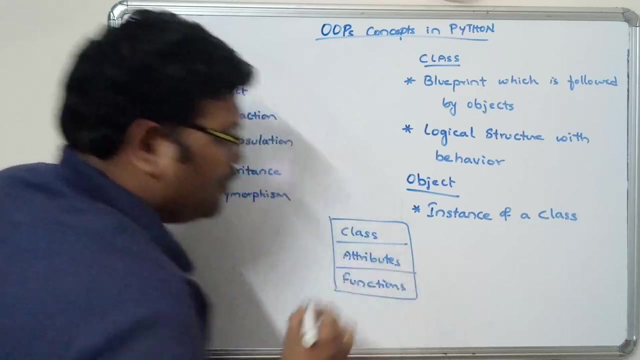 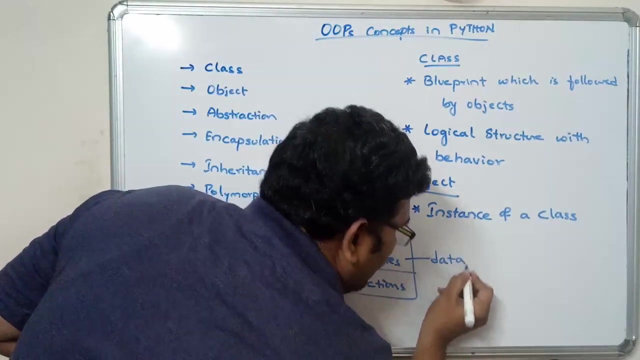 class, so object. what is meant by object? so object is an instance of a class. so here a class can have the attributes and functions. attributes and functions, right. so attributes gives the information about the class, this we can call it as a data and this we can call it as a functions. so 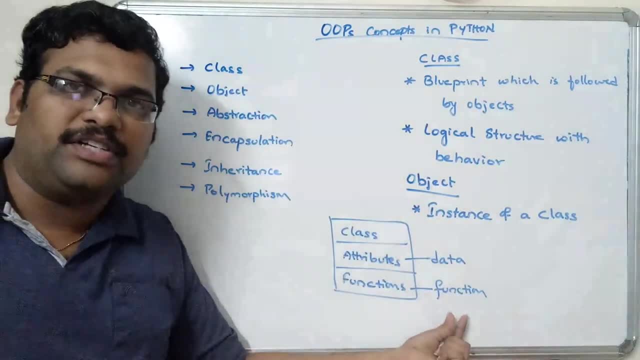 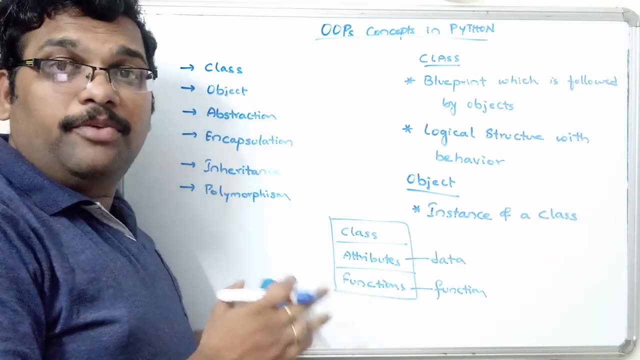 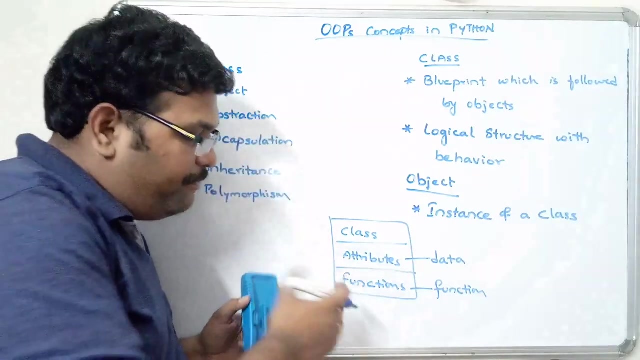 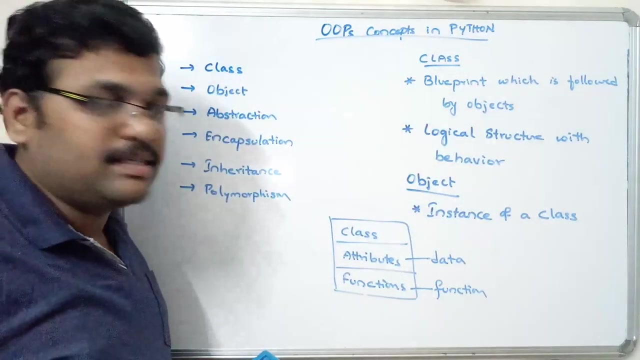 every class will be having the data and function and if one class wants to communicate with the another class, so here the communication means invoking the functions of one class to another class. so communication in is meant with invoking the methods or a functions which are available in one class with the another class, so that communication cannot be done. 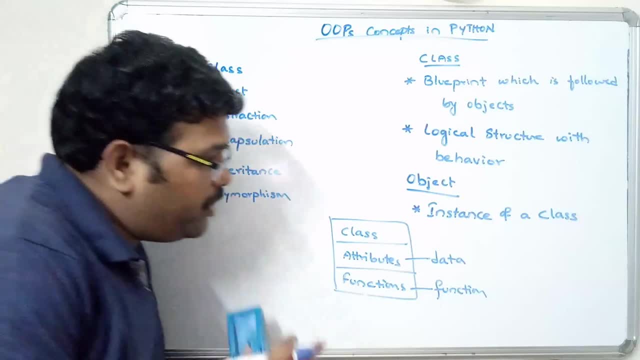 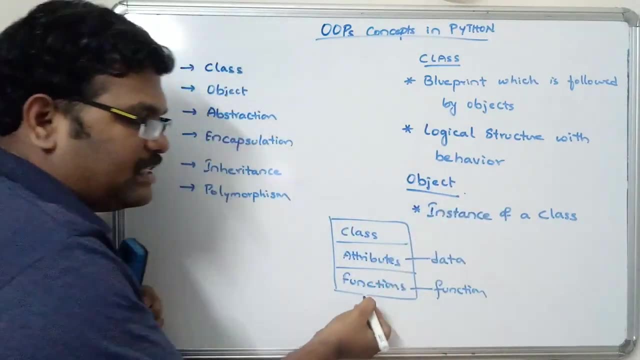 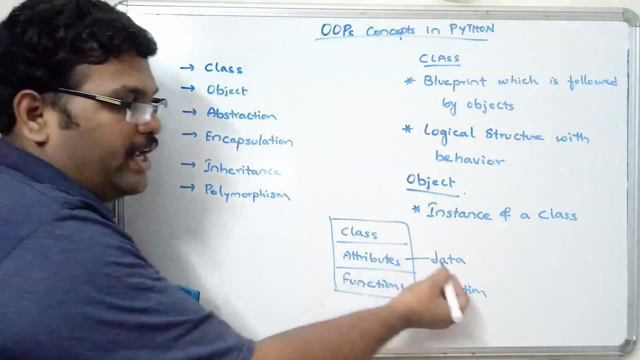 directly through the classes and in order to have the communication, that will be done only with the help of objects. so that means so with the help of object only we can access the methods of a class. with the help of an object only we can access the attributes of a class, so data and 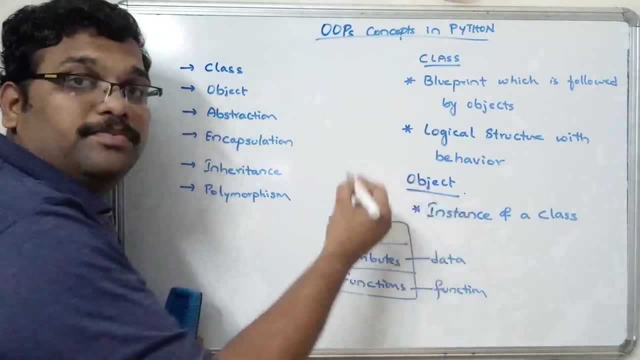 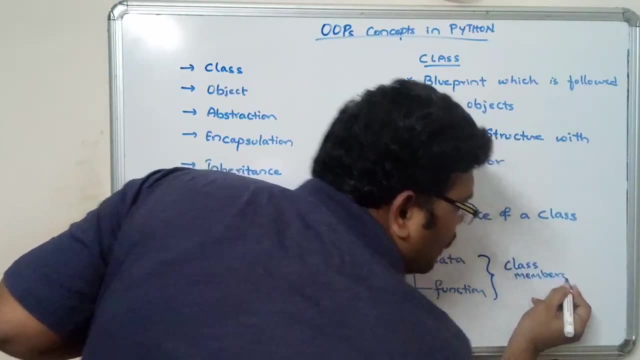 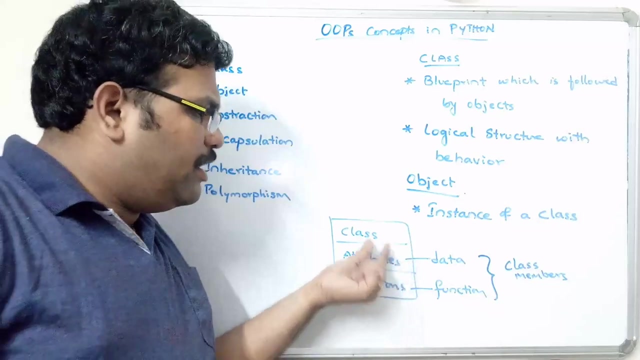 function. we can access the data and function to the help of object. so this we do. we call it as class members, class members, so every class will be having the data and a function right, so optional. sorry it may have one or two classes, but basically we're talking about hunting a class or a class. 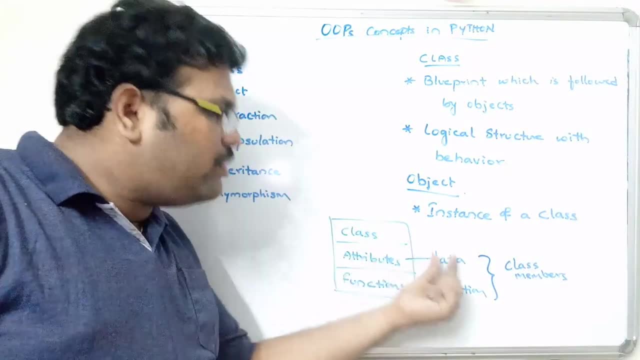 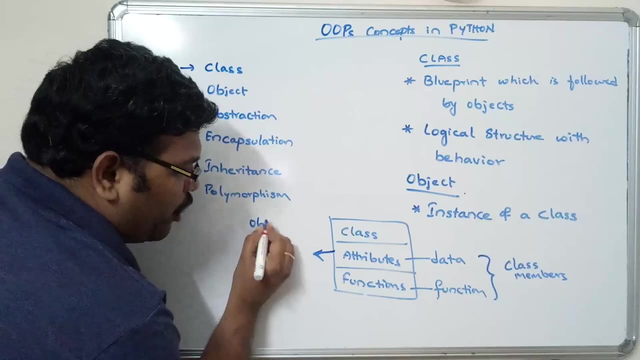 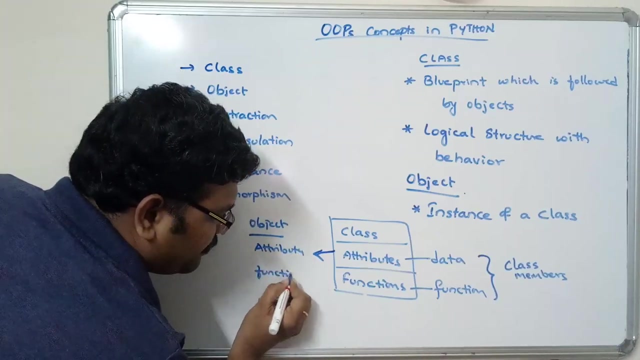 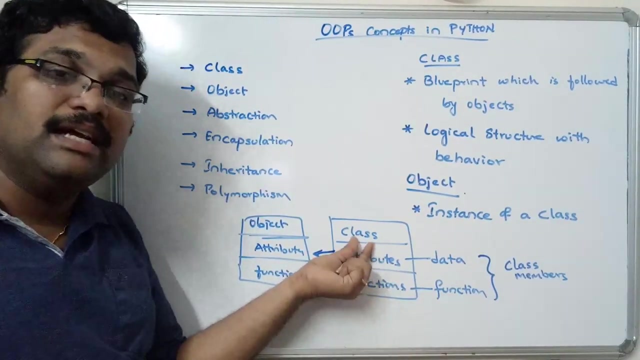 have an attributes and it may have a function, but class can have the data and a function that means a class: members. so whatever the instance we are creating for this class that is called an object, it may also have an attributes and functions. so, whatever the attributes and functions we are created for this class, all those attributes and 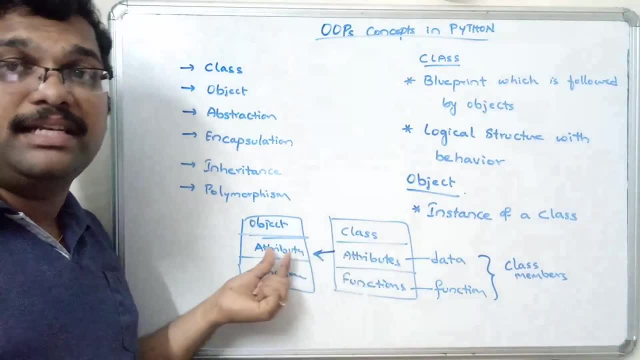 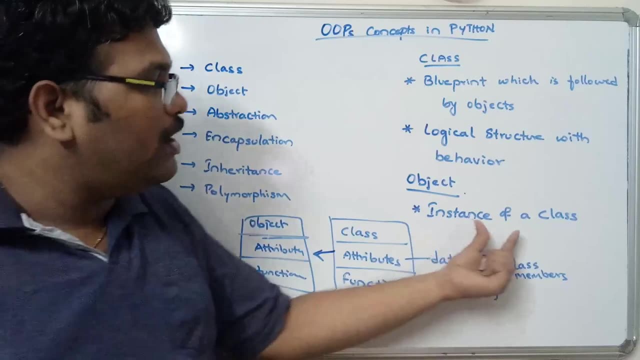 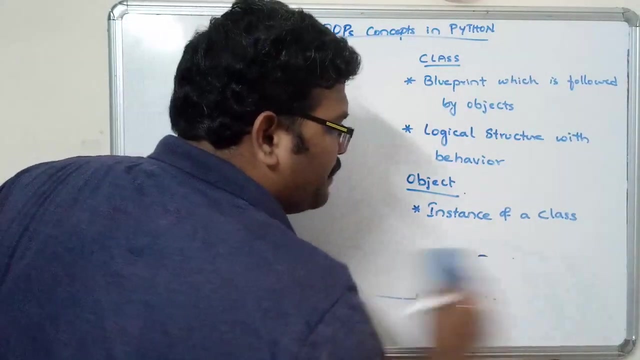 functions are available for this object also, that particular instance also right, so we can access the attributes and functions with the help of object. so that's why we call it as an instance of a class, reference to a class. so every class may have multiple objects every class may have. 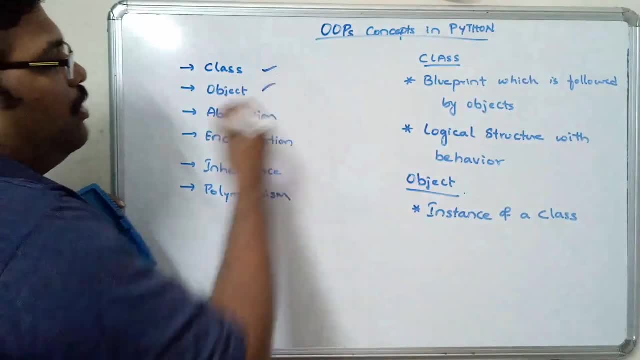 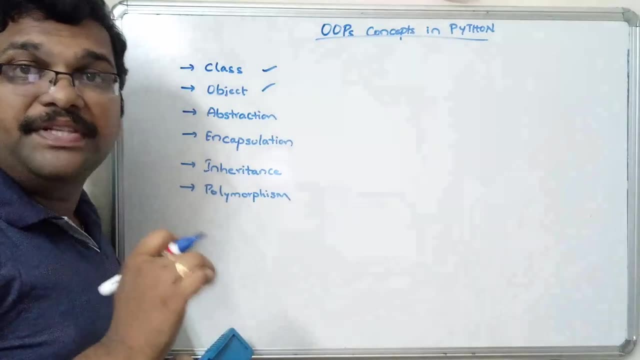 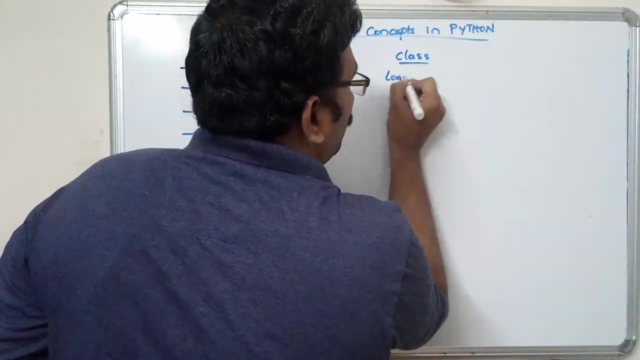 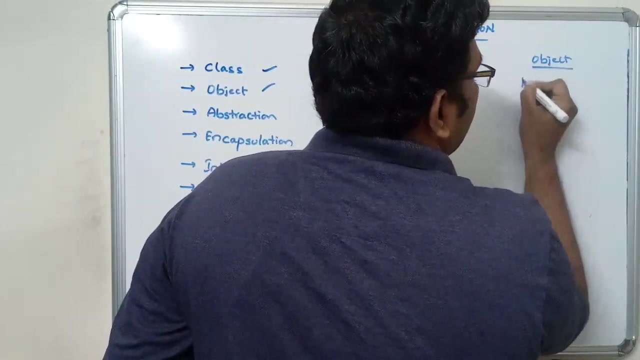 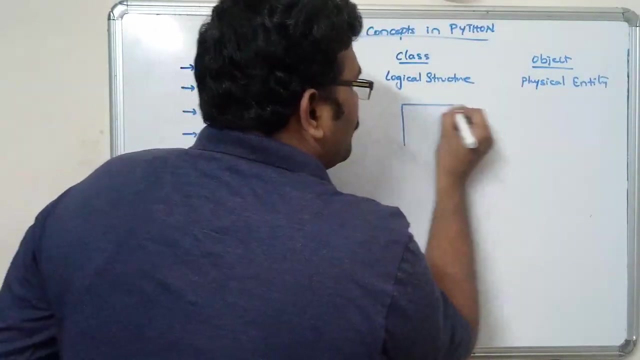 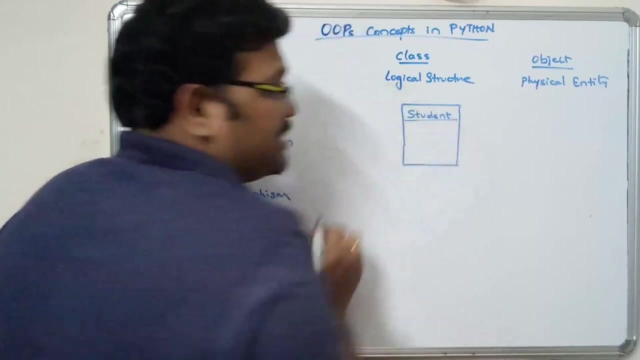 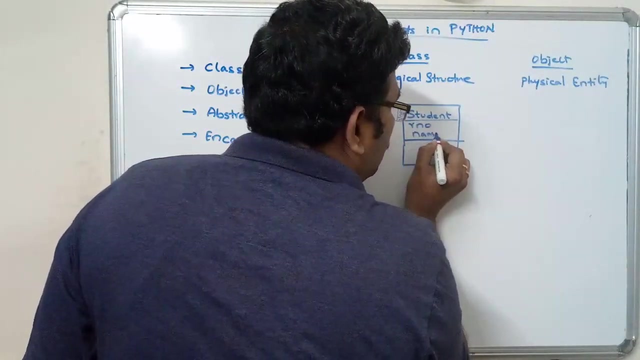 multiple objects. so i will give you an example for class and object. see: class is a logical structure and and and object is a physical entity. so class logical structure, object, it's a physical entity, right? let's see an example. student is a class, student is a class. a student can have a roll number. name to: 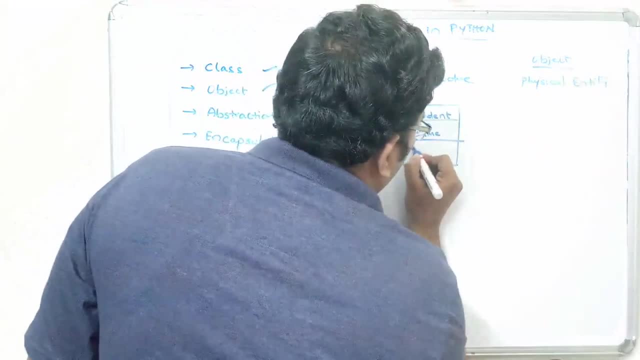 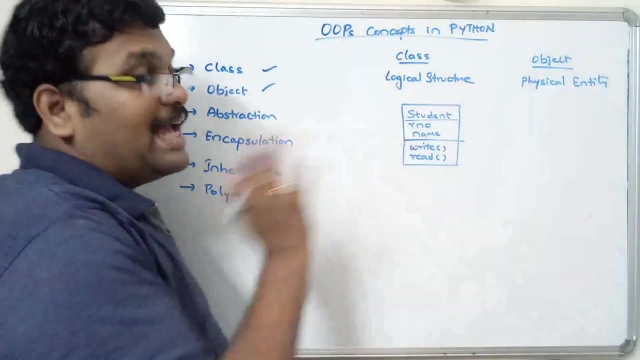 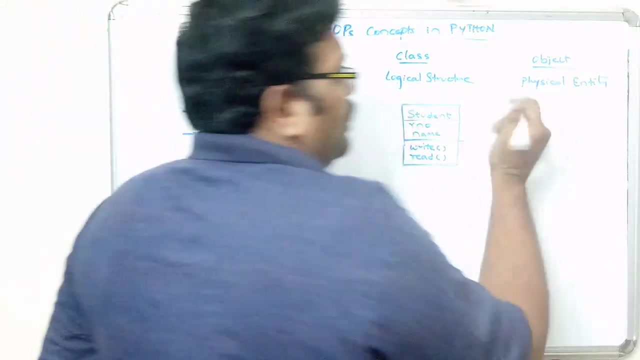 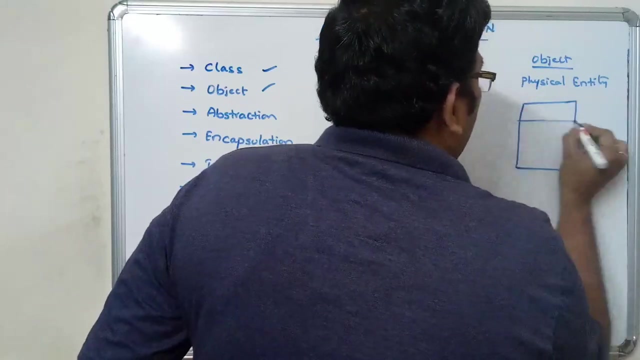 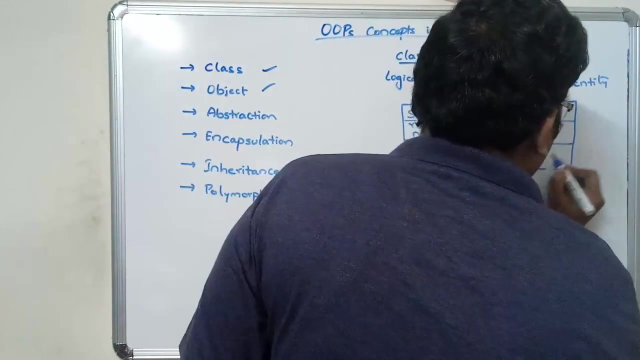 data, that means the two variables and functions. so a student can read and student can write for two functions. so this is a gas and every student must follow the blue line blueprint, right? so here see some. ABC is a name of a student that will be an object. here, right, some 1, 2, 3. 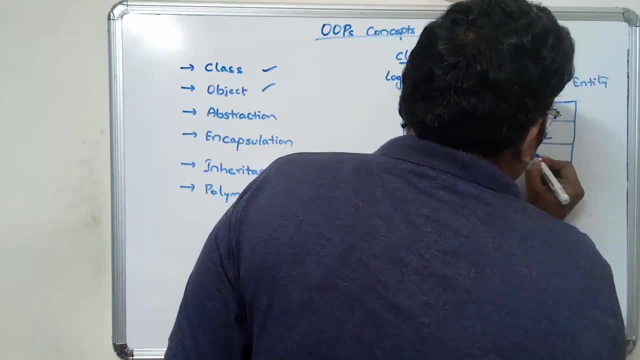 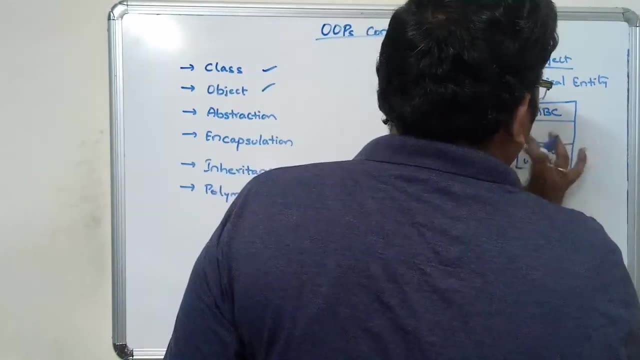 and name is ABC and some real function and a right function. so here also will be some class name and some real function and the right function. so here also will be be having that where it's same thing- our number, name, and also we can have a one. 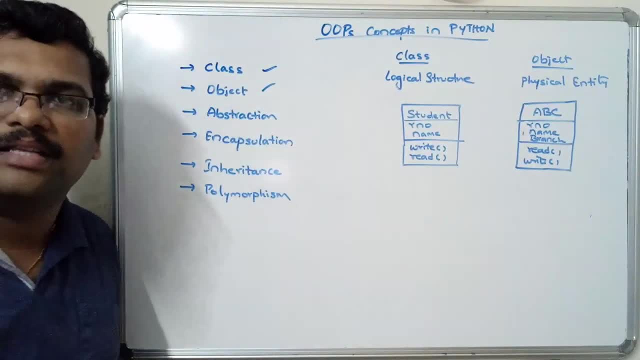 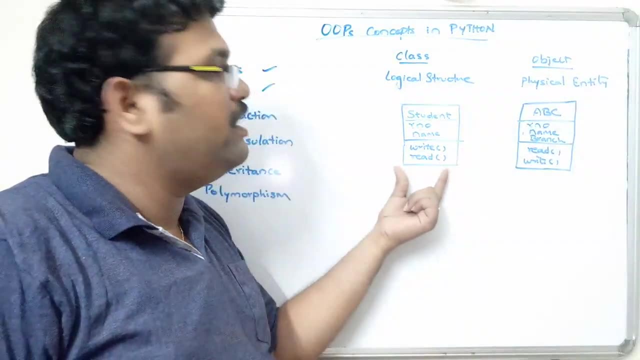 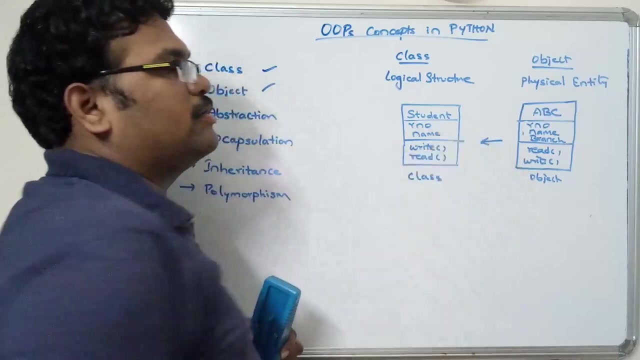 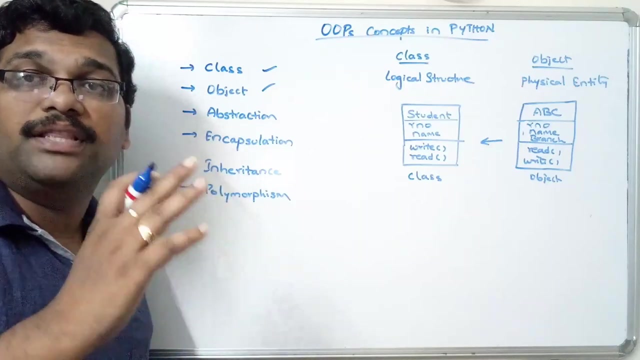 more function branch. okay, one more function branch, but this, this student, I mean this object should follow the blueprint of the corresponding class. so this is called a class and this is called an object, object of this student, right? so if our class is having around the 60 students we can have a class with. 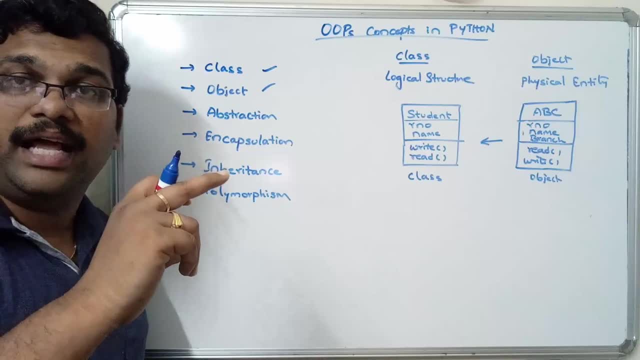 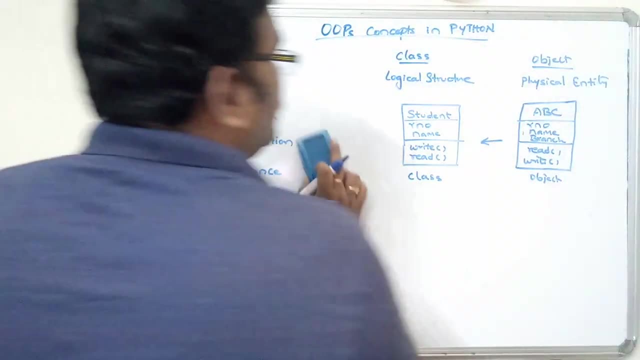 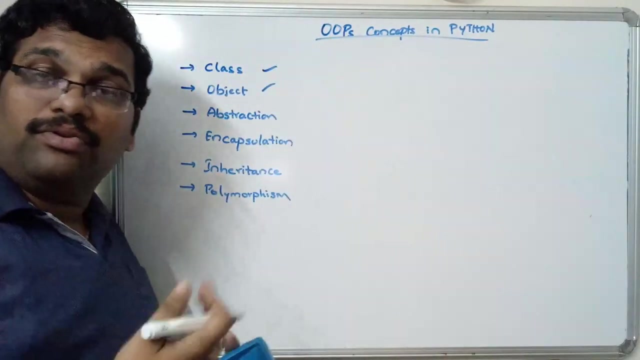 60 objects. so student is a class and it is having the 60 objects right. so hope you understood this one right. next, coming to this abstraction. so in that we will go in depth in the next session. so how to create a class and how to create an object and how to access the data and function from the class right. 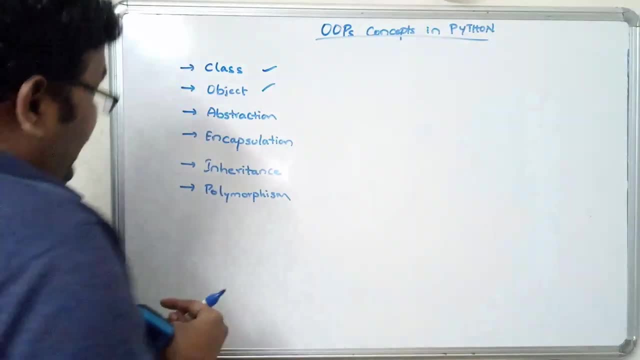 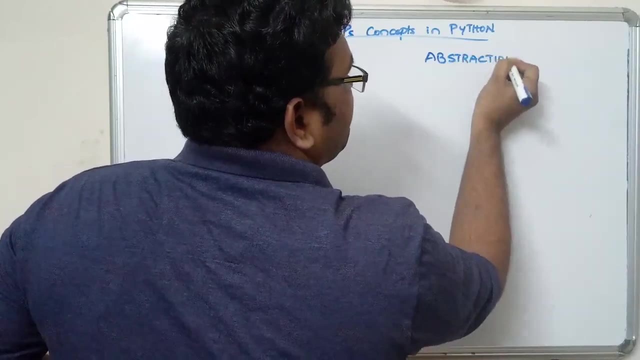 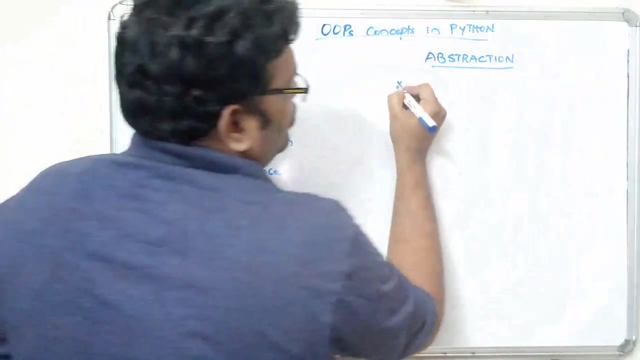 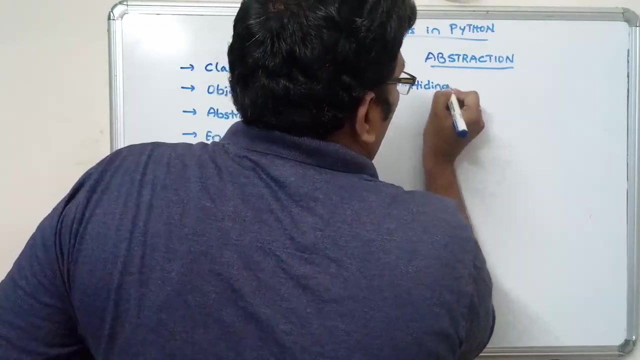 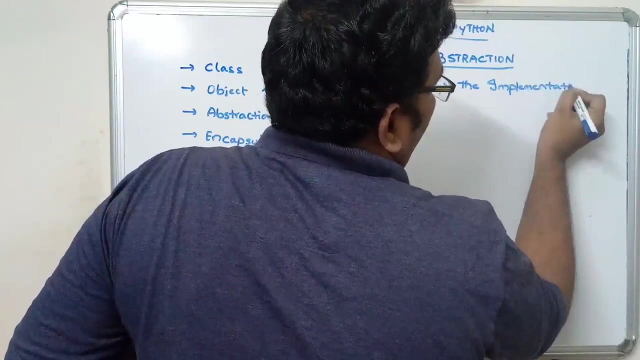 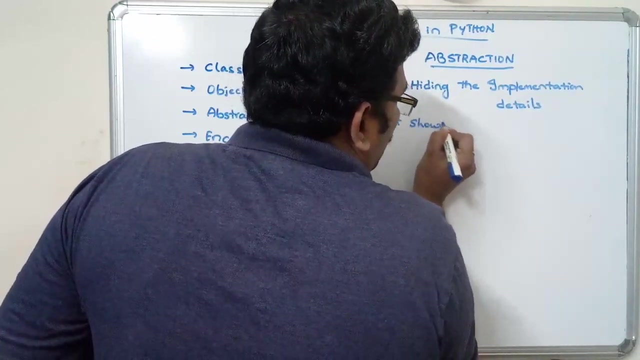 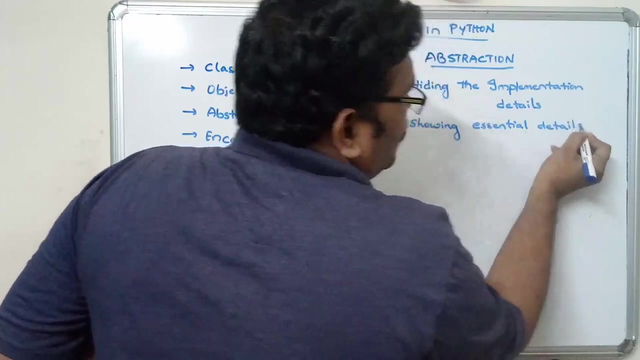 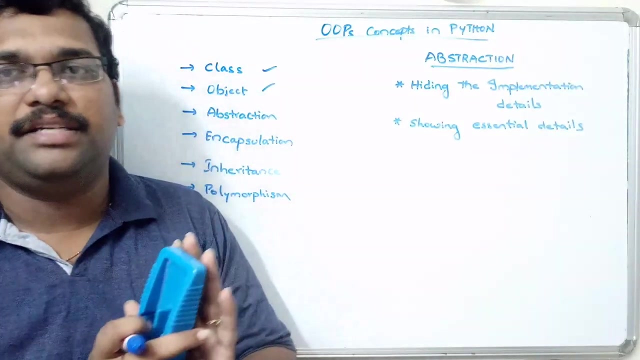 so that we'll see in the next session. next, abstraction: abstraction means hiding the implementation details and showing how we buildacas like admins, algebra factor, and so this is. this is abstract, so we hide the implementation for but we only show the essential. for example, if you over the mean a software, we don't know what are. 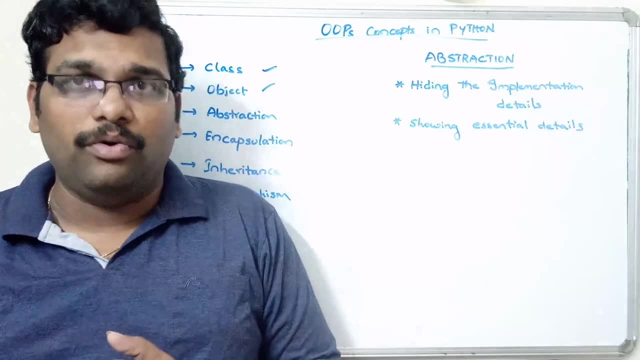 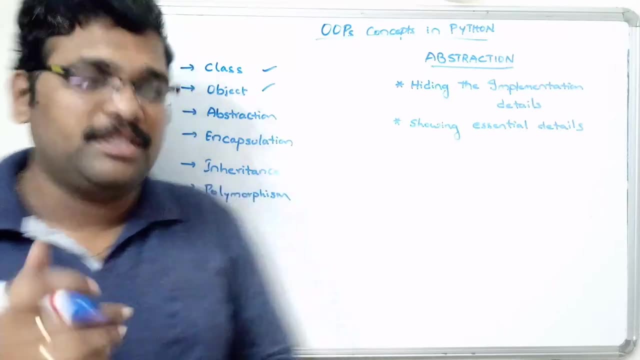 the function implemented. two: shows you the tomorrow of life structure. run the operating system right, or or any software. so just, we'll install the software. that means we will install the dot exe file, but we don't know what are the, what are the files and how the 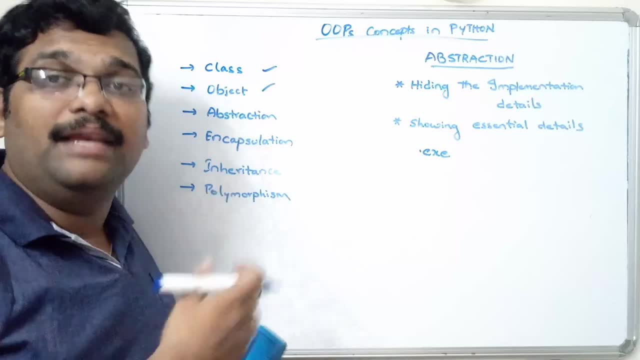 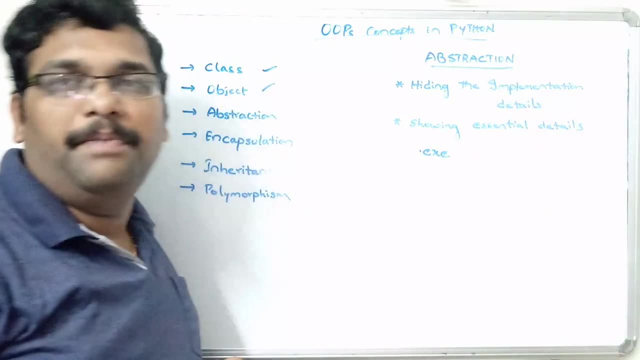 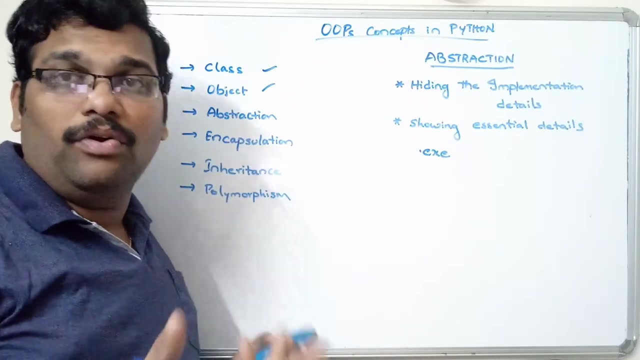 software is implemented, so that means it will hide the implementation details. all the implementation details will be hidden right. only the exe file will be visible to us. so if you install that exe file, that particular software will be start working. we don't know how, how that software 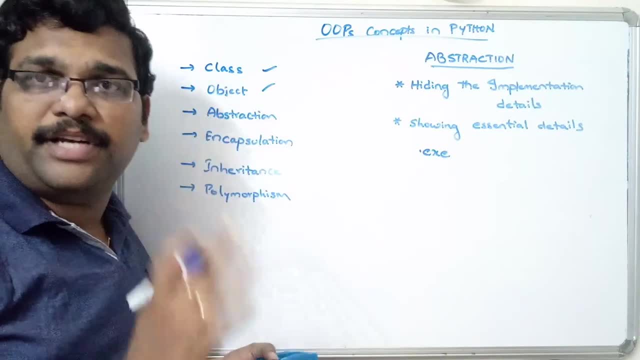 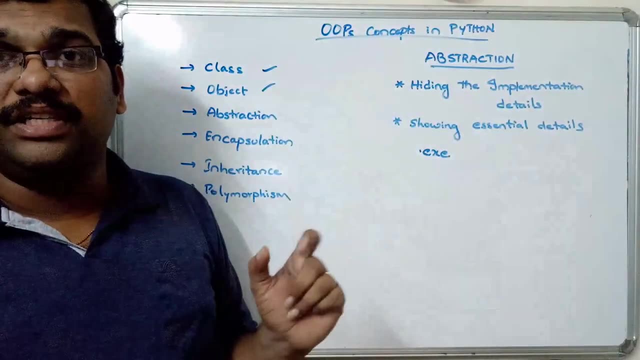 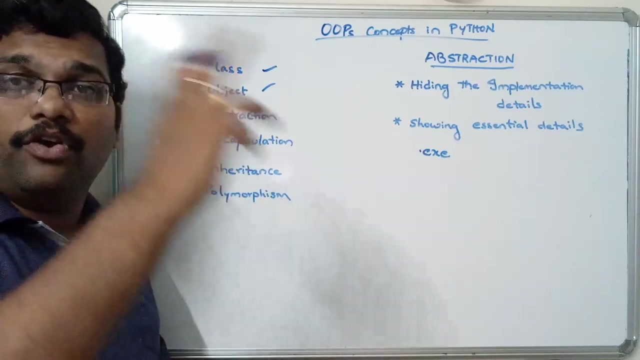 is implemented, right. so that's a small example for this abstraction. so implementing the hide, i mean hiding the implementation details, only showing the essential parts. so this is called an abstraction. so this can be implemented in object oriented concept. so in depth we will go with the another class, right? so next encapsulation. 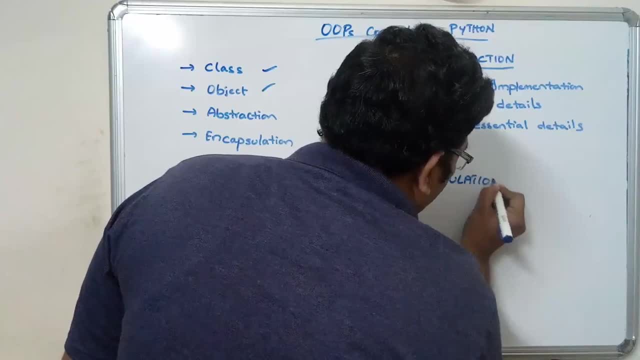 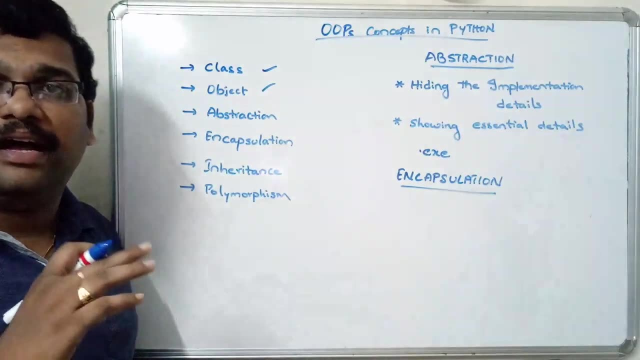 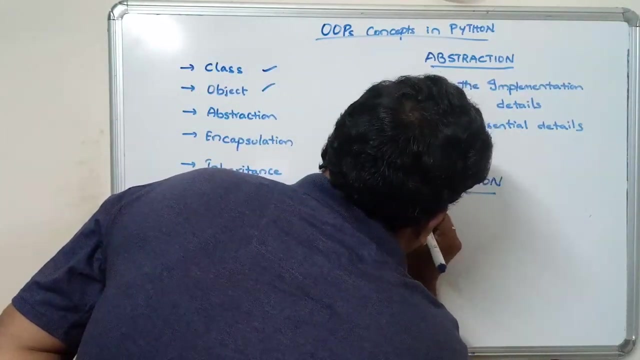 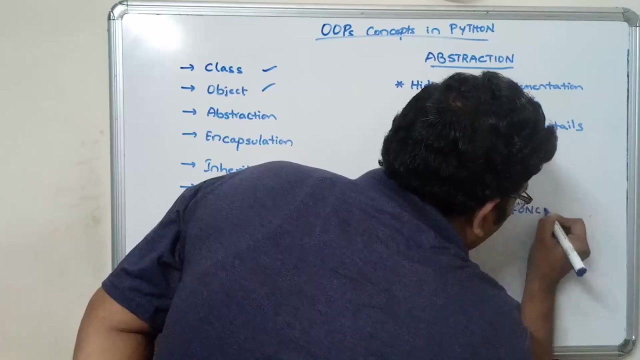 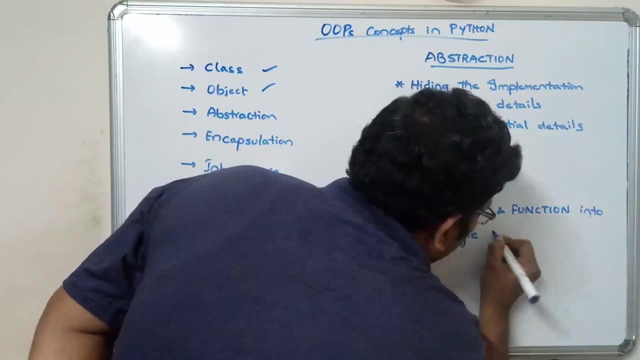 encapsulation, so here wrapping up of data and a function in a single entity, so binding data and function into an encapsulation. so here: wrapping up of data and function in a single entity, so that we can call it as an abstraction, i'm sorry. encapsulation, so here: 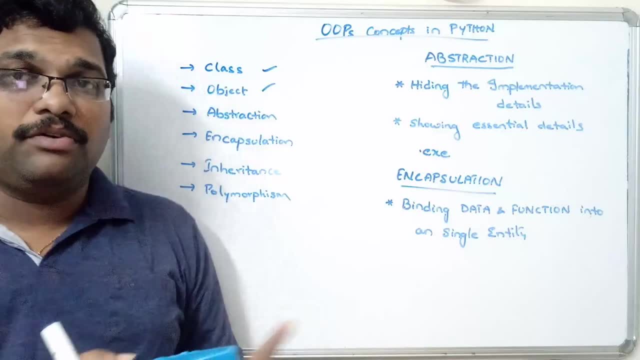 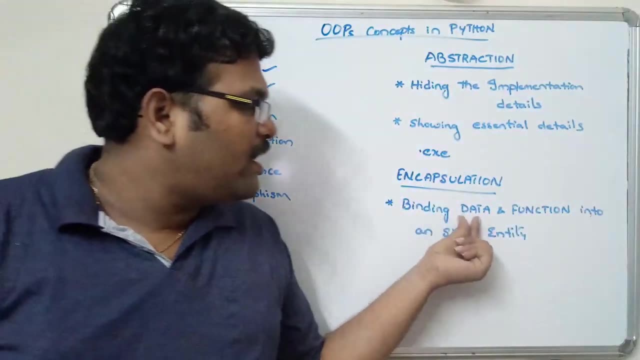 just now. i have said that a class can have a data and a functions. so that that's what i'm saying: the binding up of data and functions into a single entity that we call it as a class, right? so that's why, that's how we can achieve this encapsulation. 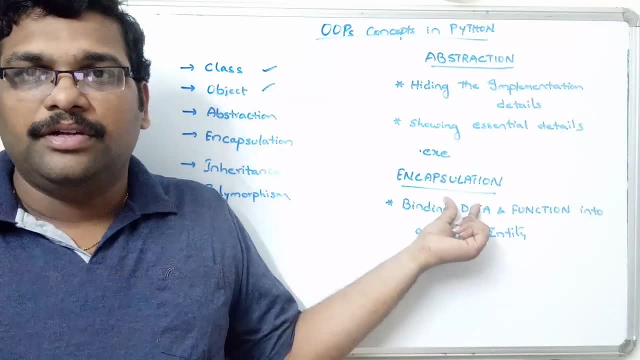 so by using the access place function, it is removing data directly from thatЕnc npc group, parts from some subgroups, because it is not science, because it is eyes, so we can extract that. six the access specifiers: so there are three access specifiers, so public, protect and private, so these 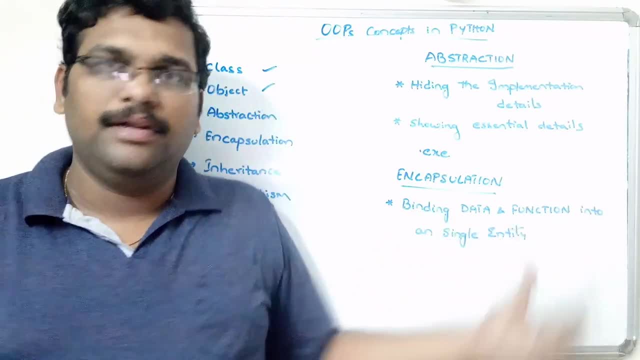 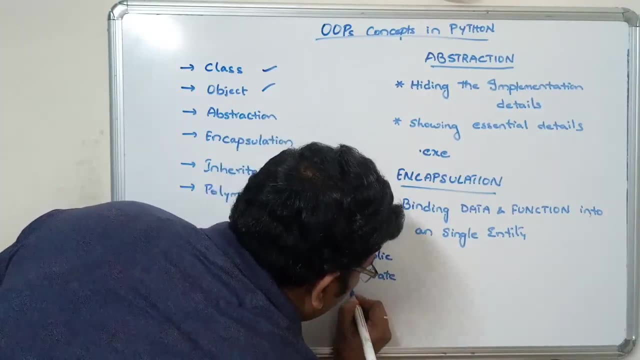 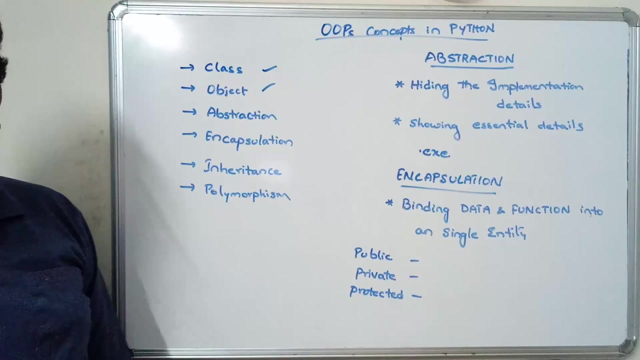 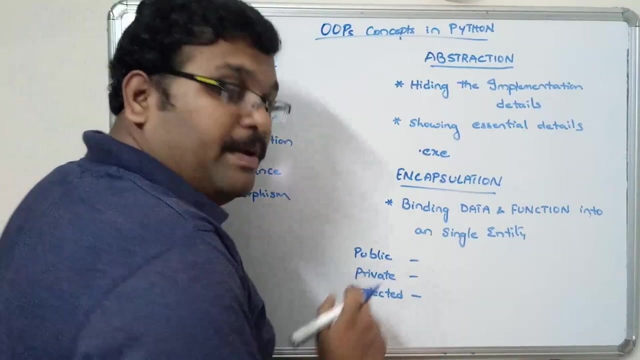 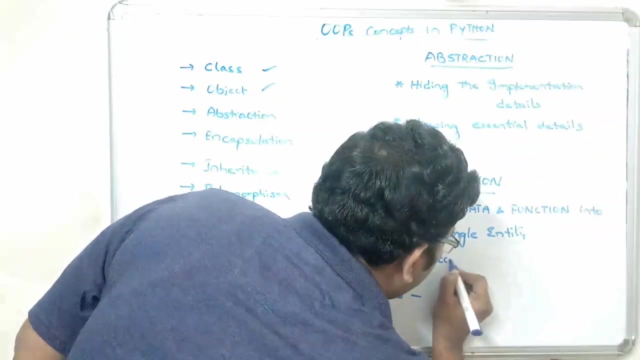 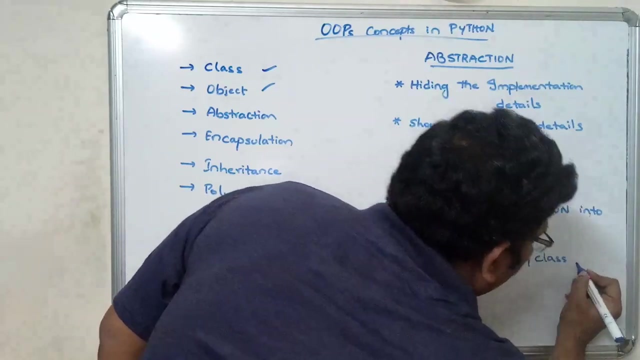 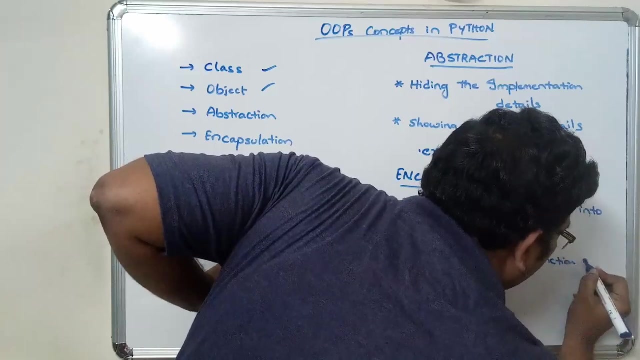 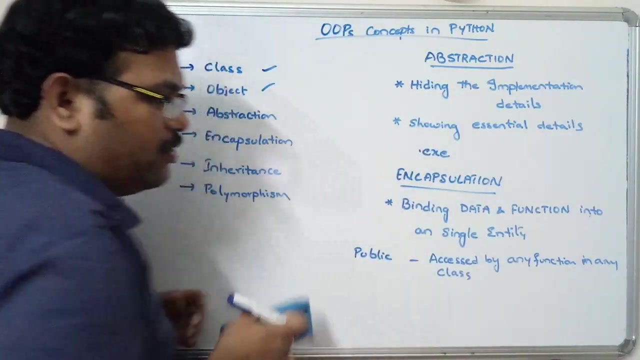 access specifiers can be applied for these data and functions right. so one is a public, private, protected, public, private and protected right. so public means whatever the data and a function available in one class that can be accessed by any class, any function in any class. right. so if the data and function are specified with the public, 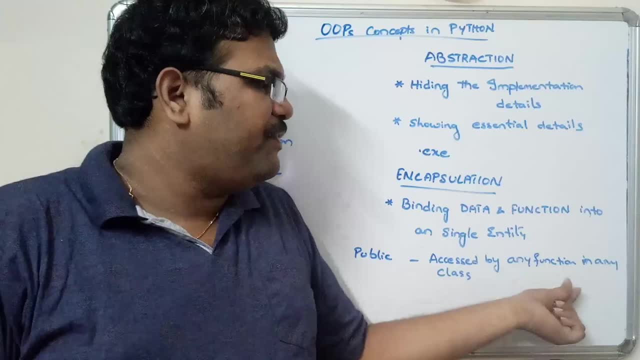 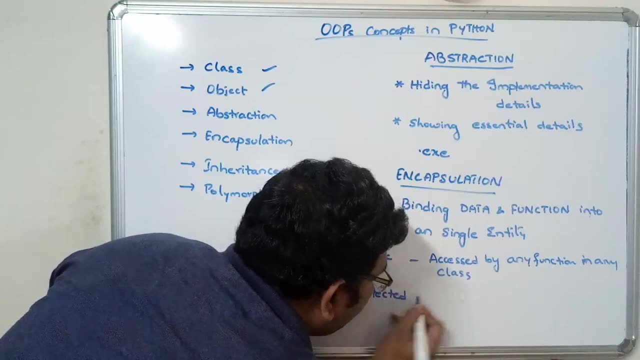 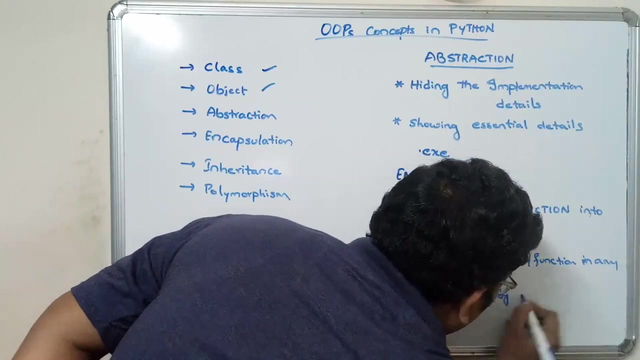 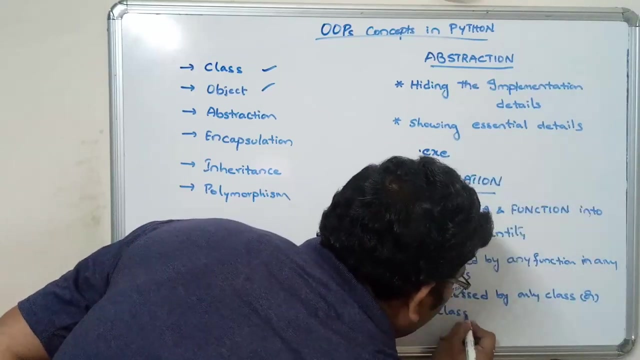 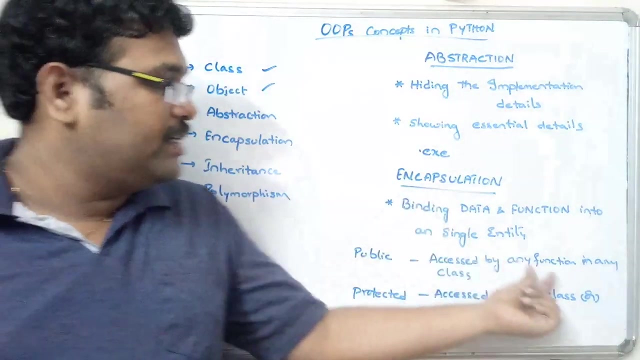 those data and functions can be accessed by any function in any class if it is a protected. if it is a protected, so it can be accessed by only class where it was declared or inherited. so in which class we are declaring those data and functions? that class only we. 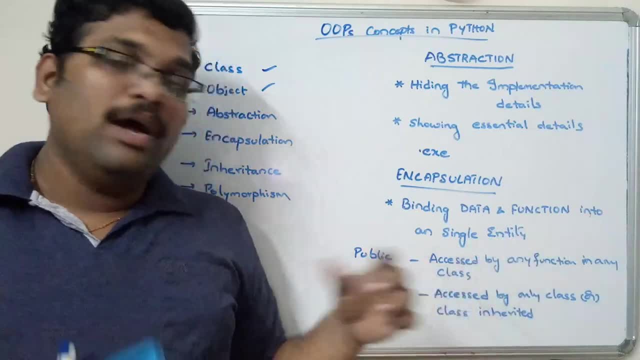 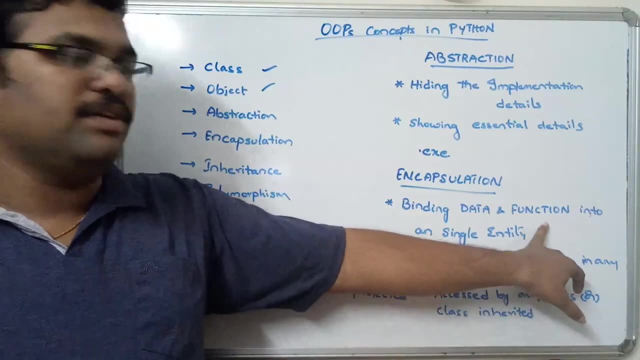 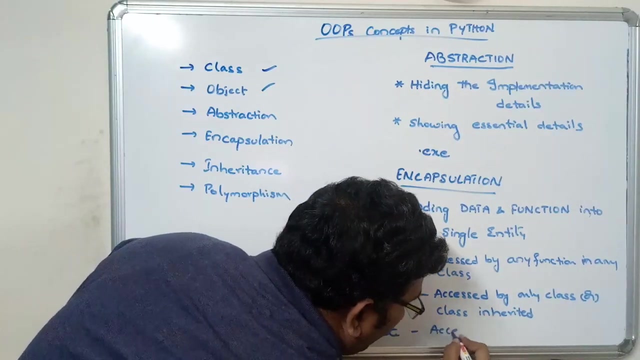 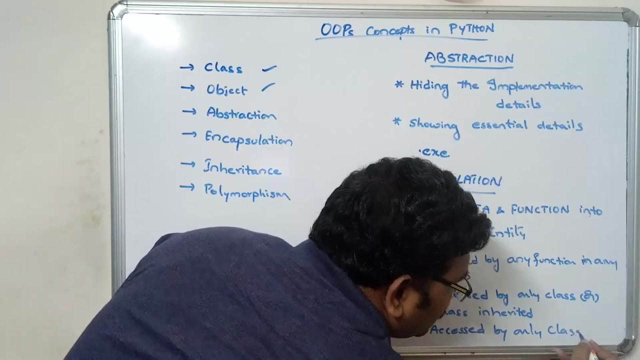 can use those data and functions or whatever the class which is inherited from the base class. in that class also we can use the data and functions. and if it is a private, these data and functions can be accessed by only that class, only class in which this data and functions are declared. but also we 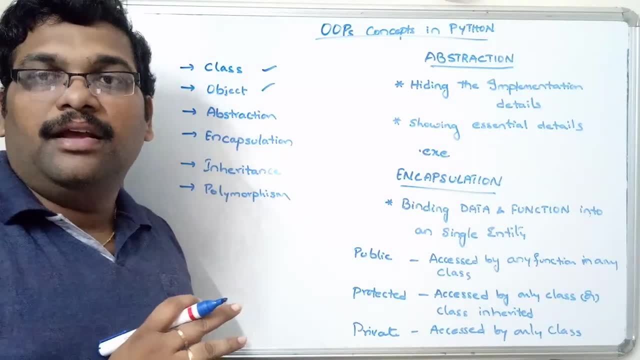 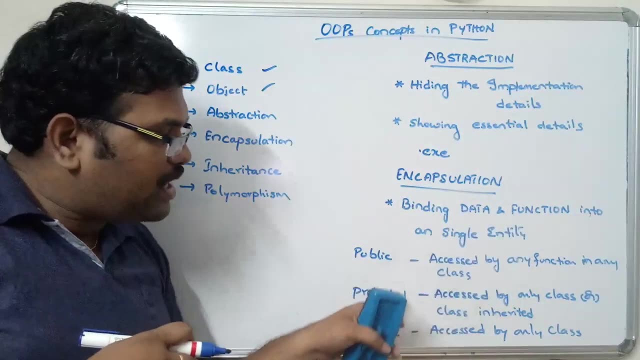 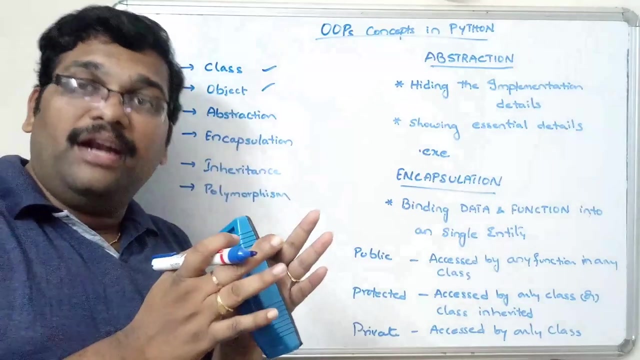 cannot use them in the inherited class, right? so we can inherit one class with another class. so here, if it is, if the data and functions are accessed as a protect, in a level protected, then they can be accessed by the class where it is declared and also the class which is. 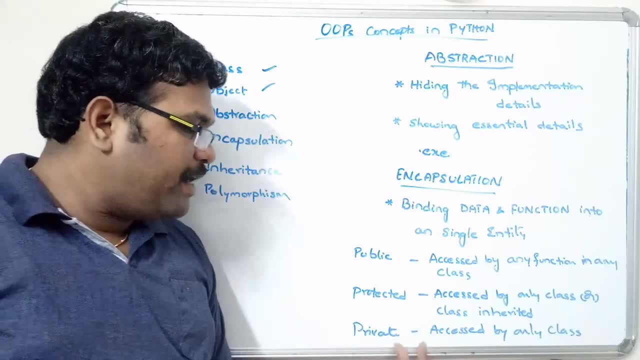 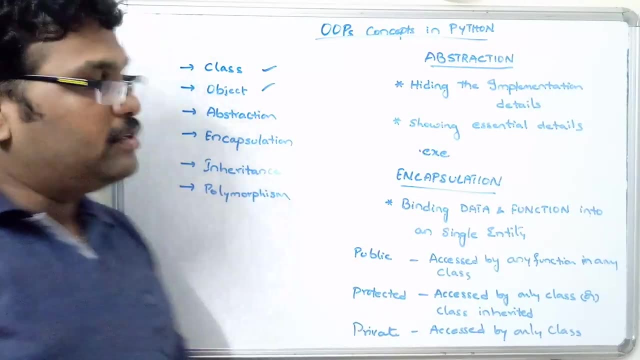 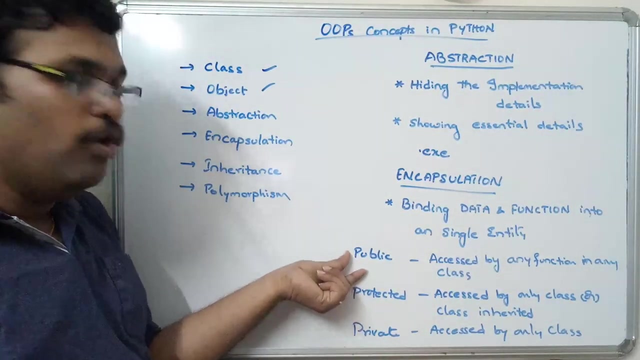 inherited from the base class, but here, if it is a private, it can be accessed by only one class. that is where these data and functions are declared right. so this is how we can achieve this abstraction and encapsulation: by using these access specifiers right. so this is called a low 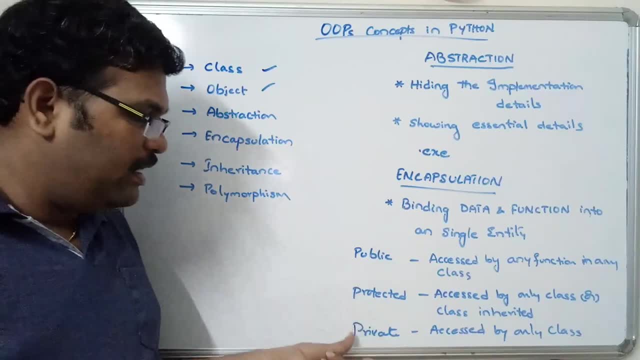 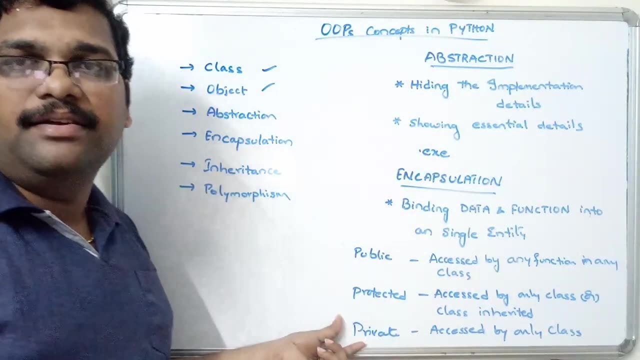 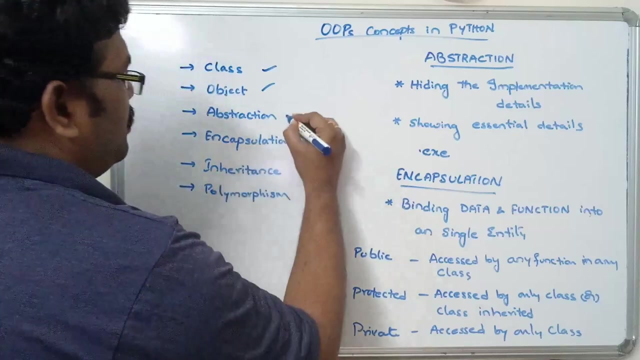 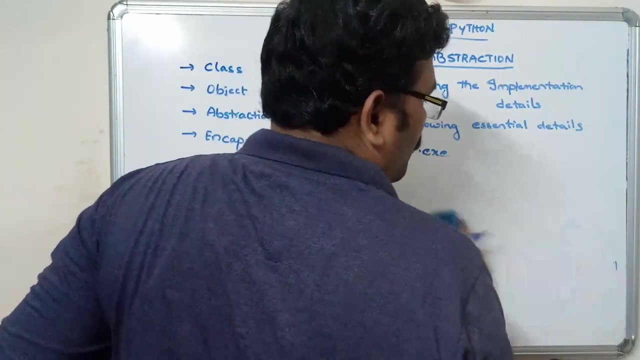 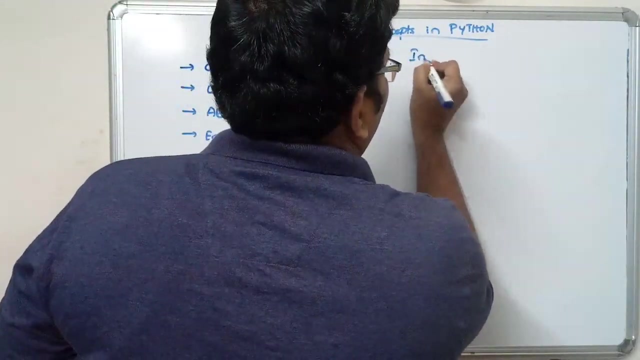 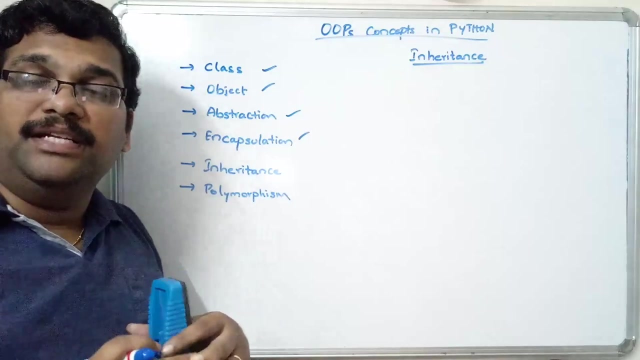 level protection data production. so this is a medium level and this is a high level data protection. so because we are restricting the privileges, we are restricting the access of this data and function right. so hope you understood. so next, inheritance concept. inheritance concept means the base class and the derived class. so 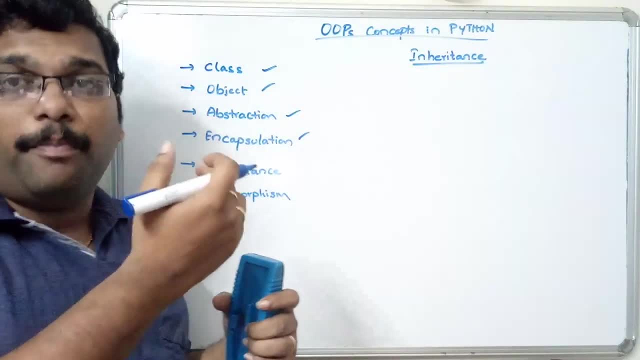 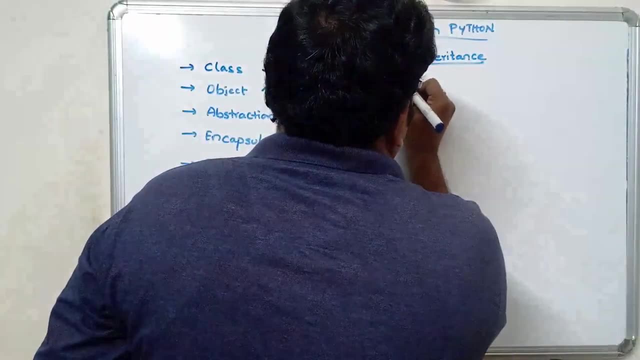 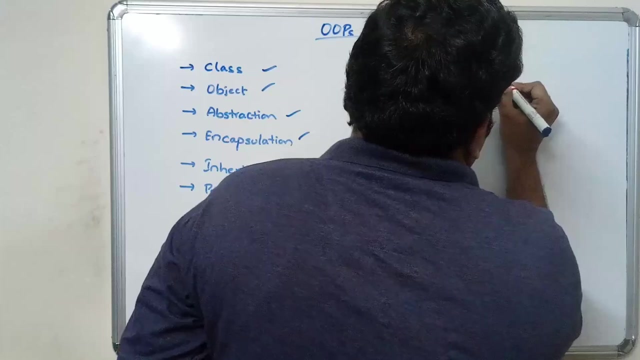 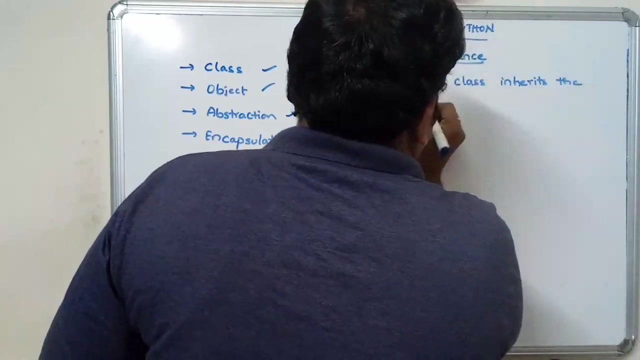 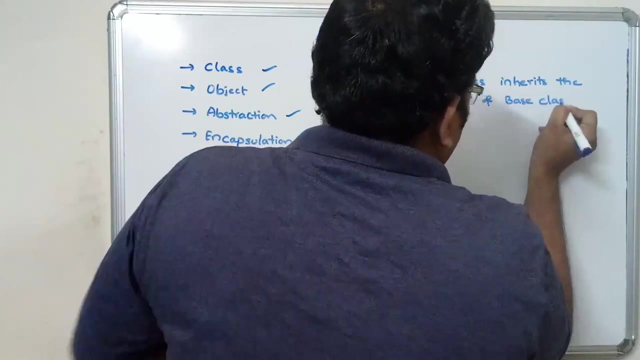 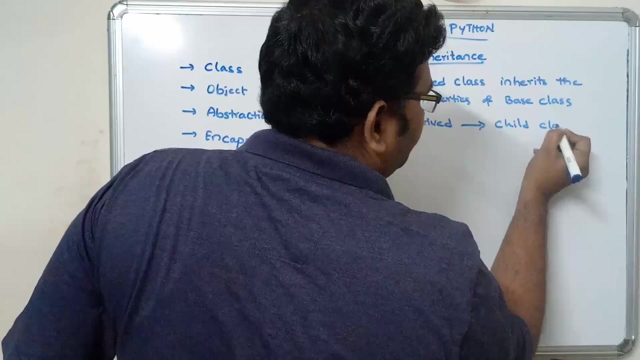 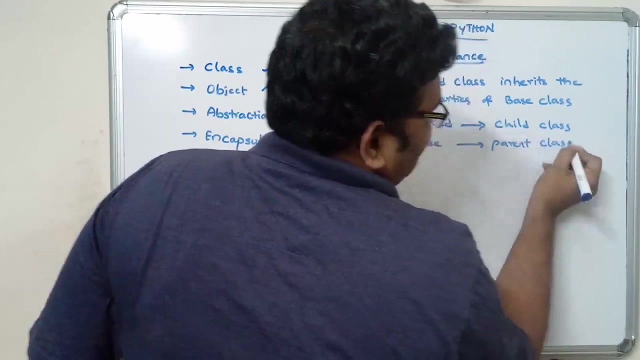 the base class and the derived class. so the base class and the derived class. so derived class can inherit the properties from the base class. so we can also call a city class in pendia. so there are class can be also called as child class. base class can also be called as parent class, so the 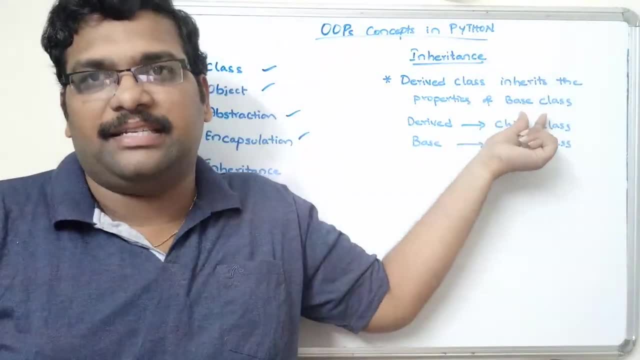 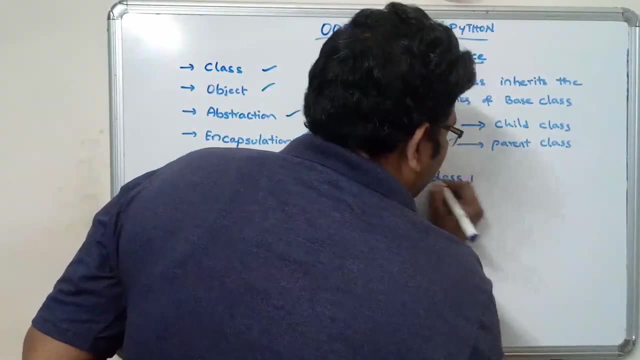 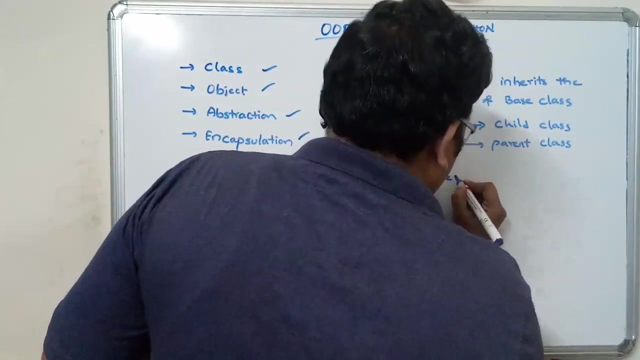 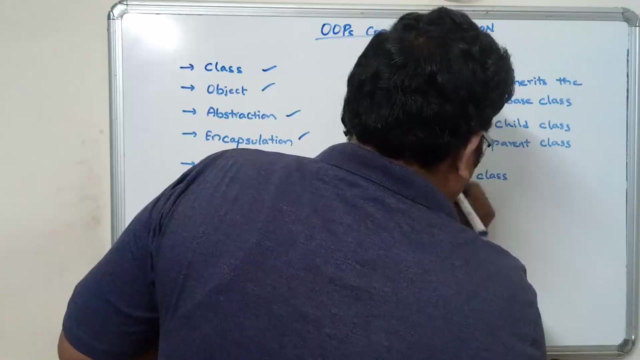 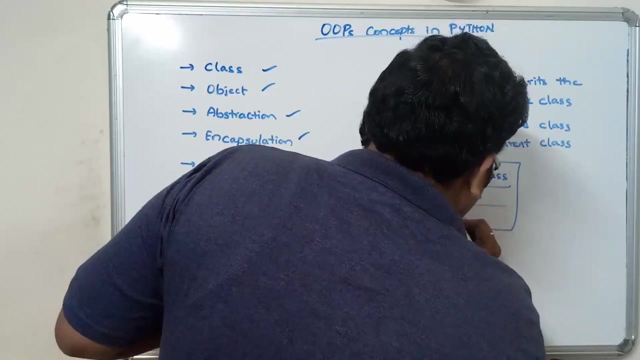 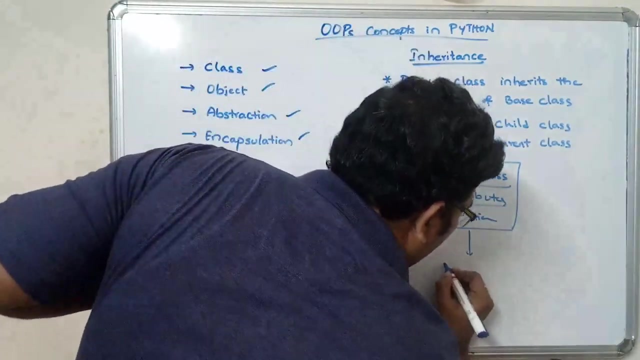 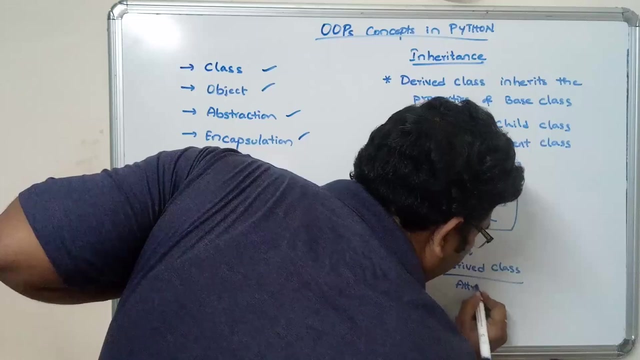 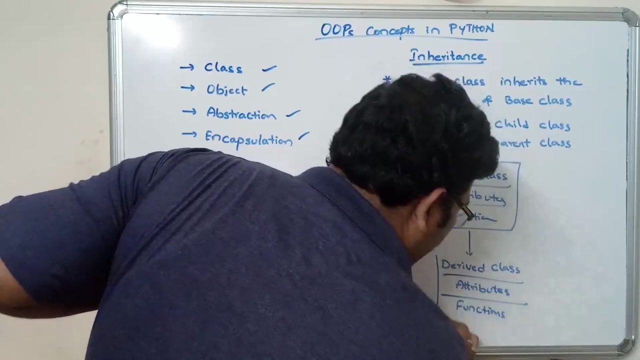 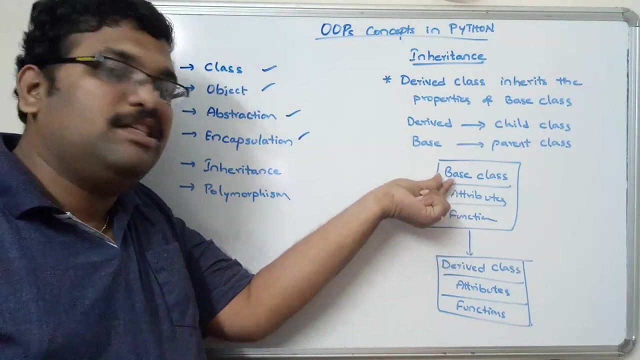 derived class inherits the properties of a base class. so what is actually meant by this one? I will give an example or we can directly write here: attributes and functions, base class, and this is a derived class. here also we are having attributes and functions, right. so whatever the attributes and functions available in this base class, 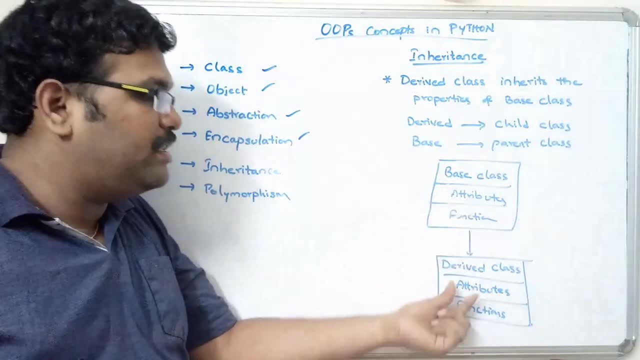 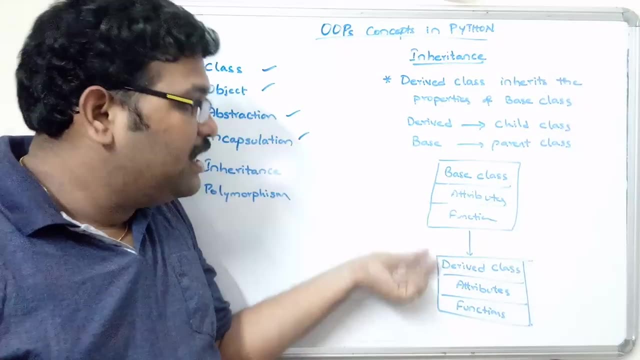 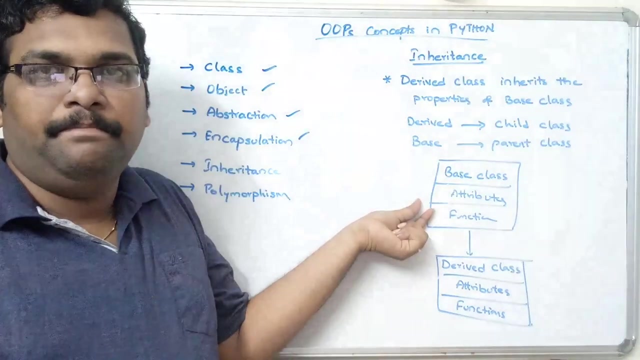 all those can be also accessed by the derivative class. so this derivative class will inherit the properties of a base class. that means it will be having. this derivative class will be having the same attributes and the same functions which we are using in the base class and in addition to 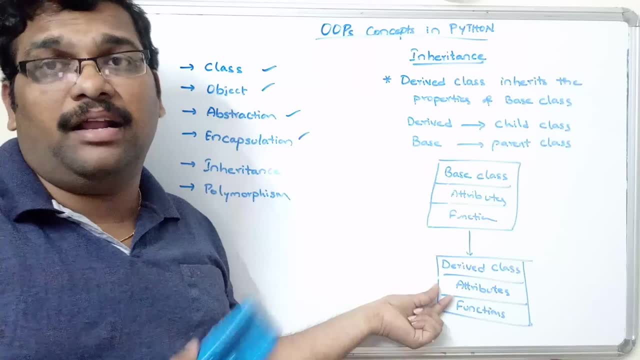 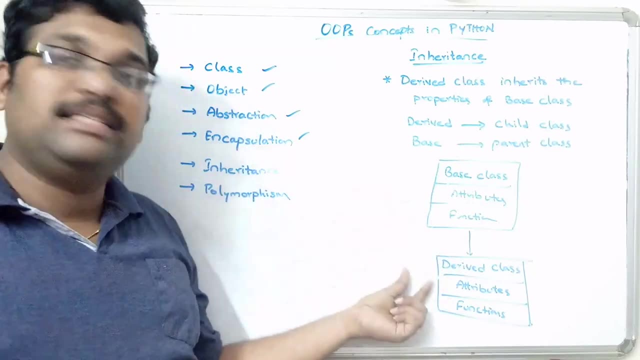 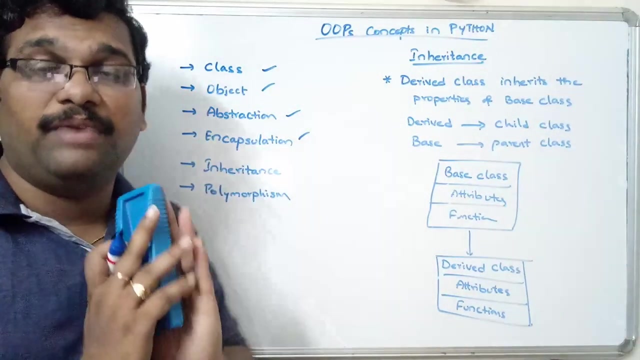 that we can have another attributes and other functions. so that depends upon the derivatives. okay, so this is a parent class, this is a child class, so child class will inherit the properties of the parent class. so, whatever the attributes and whatever the functions we have, we have declared: 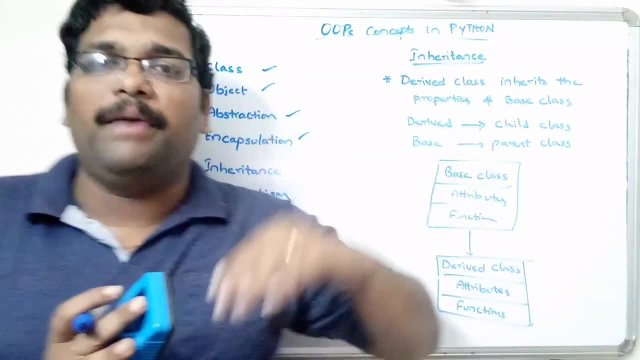 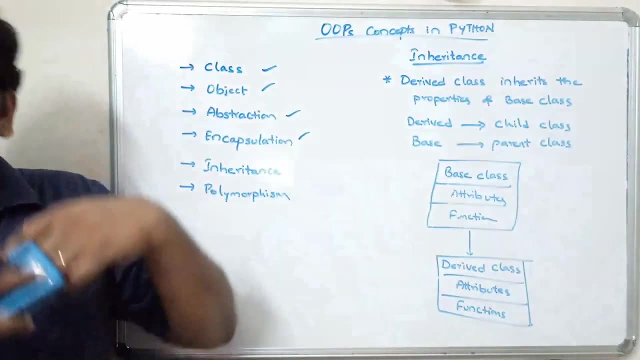 in the parent class. those can be also used by the child class itself, so that is actually called as inheritance. so here the inheritance can be used by the parent class, so that is actually called as inheritance. can be implemented in different ways, so single inheritance, so multiple inheritance. 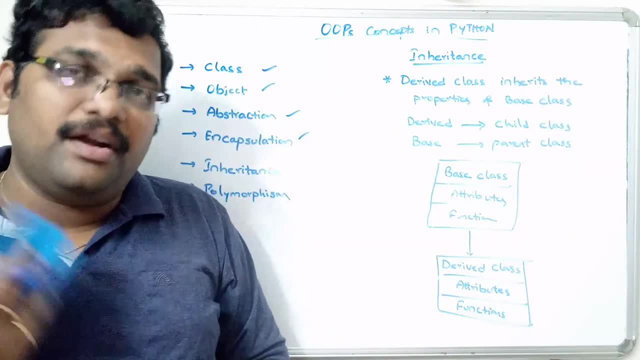 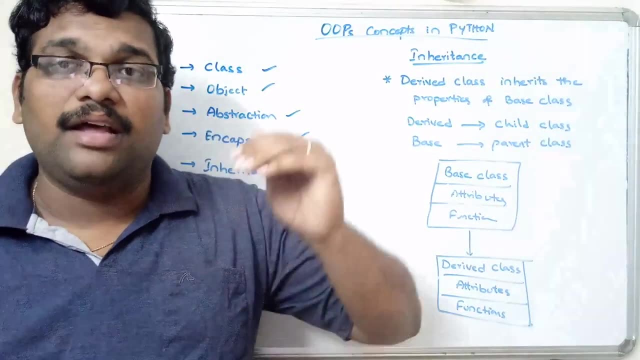 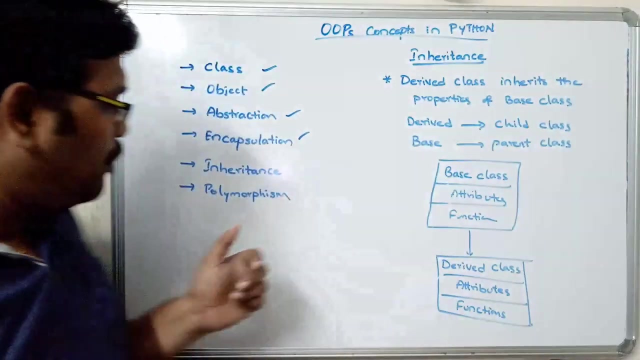 multi-level inheritance, right. so likewise a different. there are different types of inheritances, so we will see in depth in the further classes. so, but the actual inheritance concept means the acquiring the properties of a parent class by the child class, right? so hope you understood this one, and then we will move on to the polymorphism. 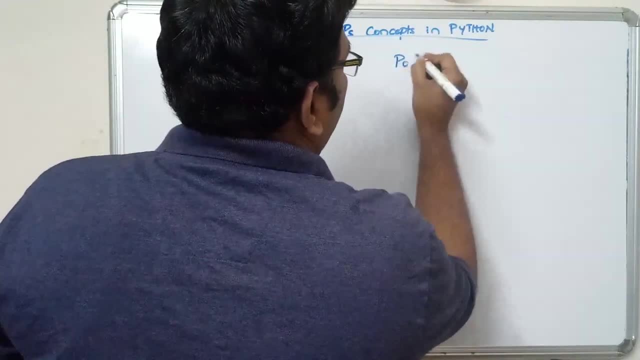 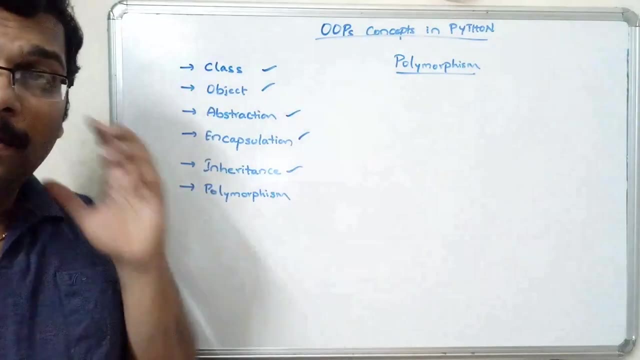 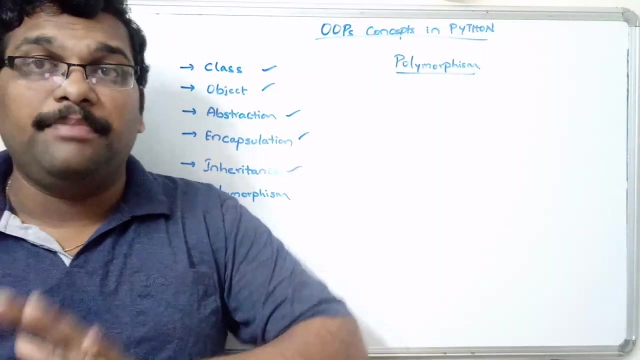 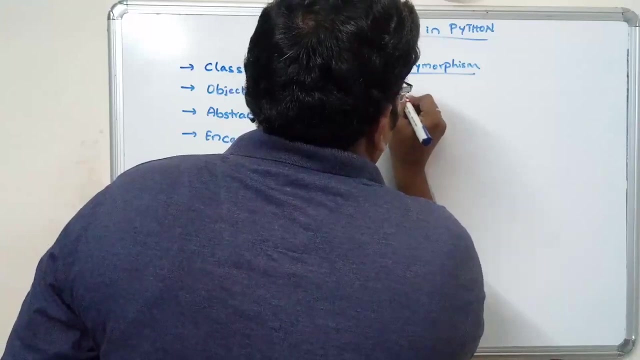 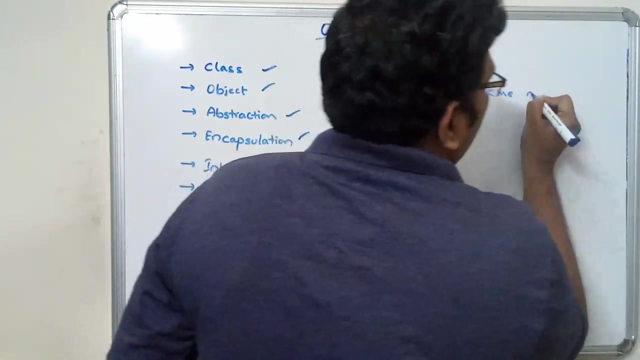 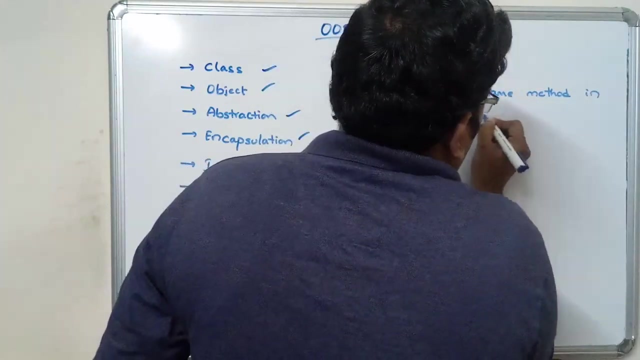 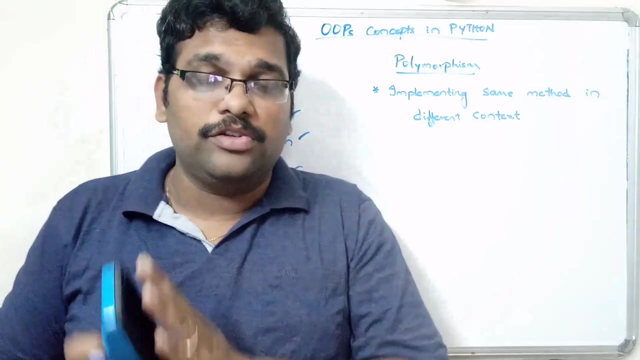 see. so here the inheritance completely deals with the classes, whereas a polymorphism will complete it, deals with the methods, right? so polymorphism means implementing, say, same method in different context, different context. so here also poly. in the polymorphism also there is a concept of inheritance. that means only in the concept of inheritance will. 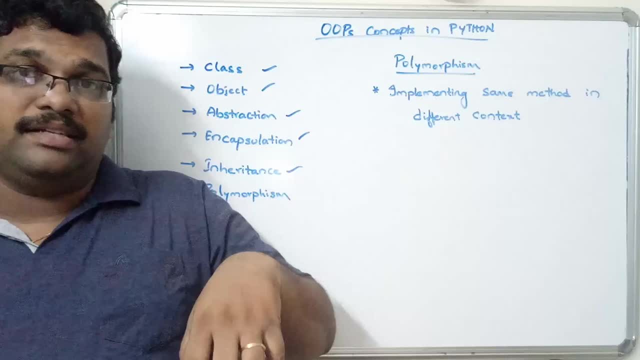 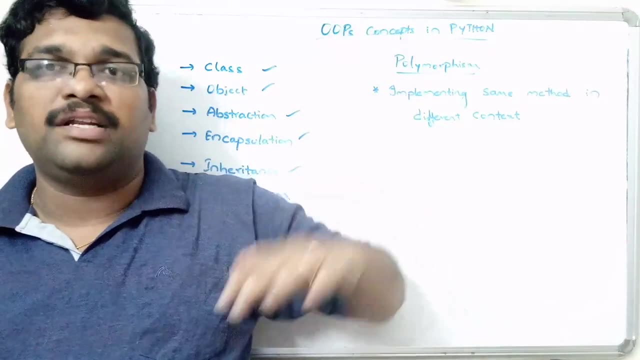 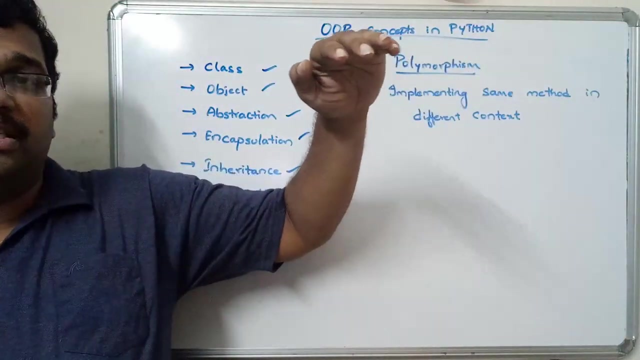 go with the polymorphism. so just now we have seen that inheritance means the parent class and the child class, so both will be having the common attributes and the common methods. because whatever the attributes and whatever the functions we are using in the parent class, all those functions, 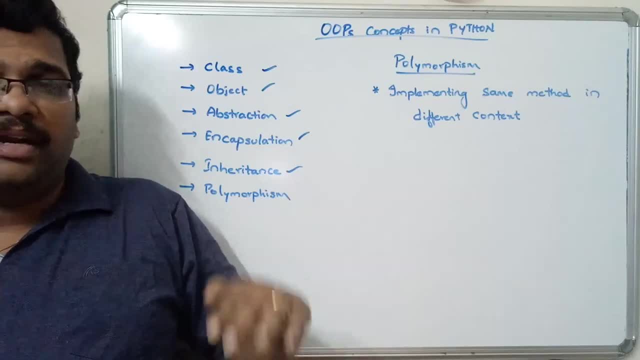 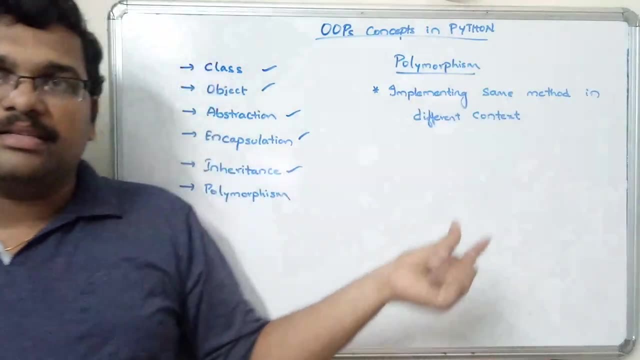 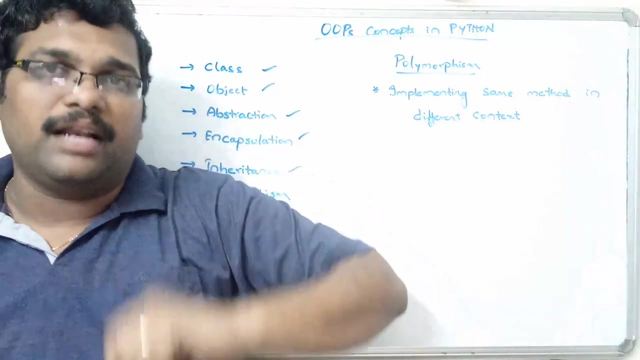 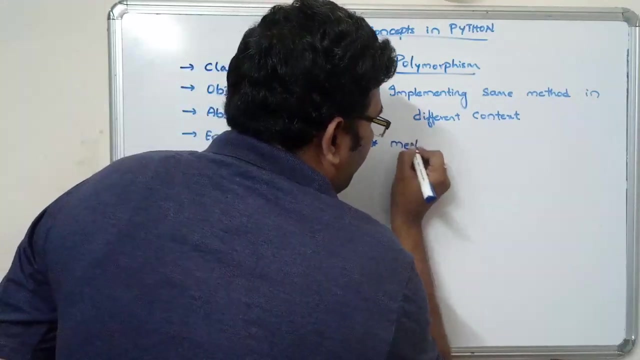 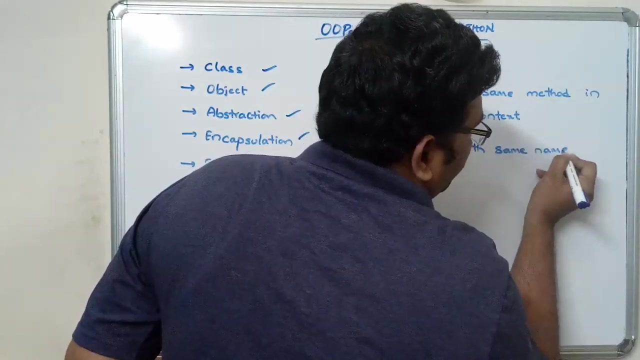 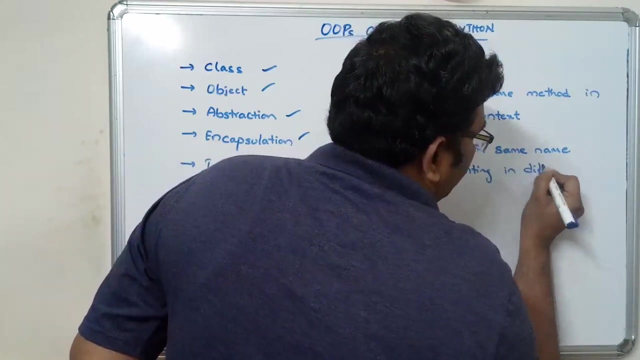 and data will be available with the object right. that means a derived class right. so here, implementing the same method in different context. so we will implement the same method in the parent class, as usual, as well as in the child class right. so here, methods with same name, implementing in different way, in different way. see, for example, if you take the addition example, add x, comma y. 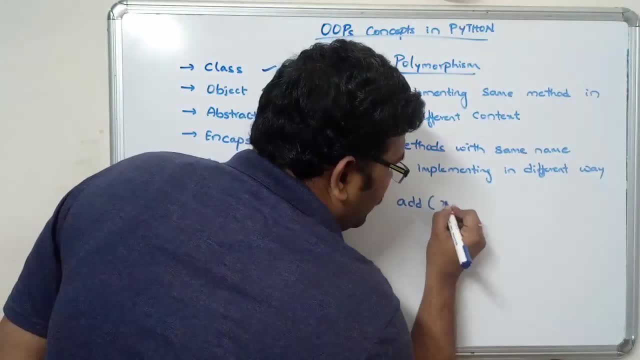 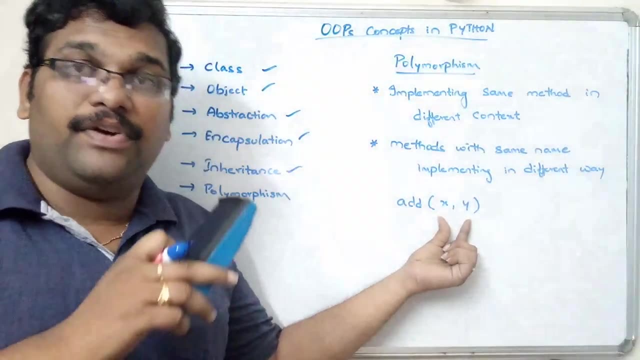 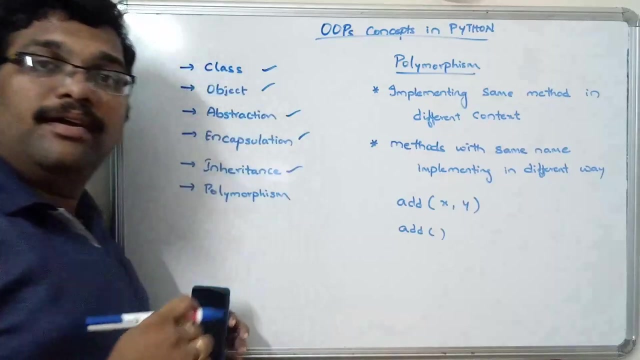 see, for example, if you take the addition example, add x comma y. so here add x comma y is a function call which takes x, y as the input. so simply we can also write add where in the function definition we can take the input values, where in the function definition we can take the input values. 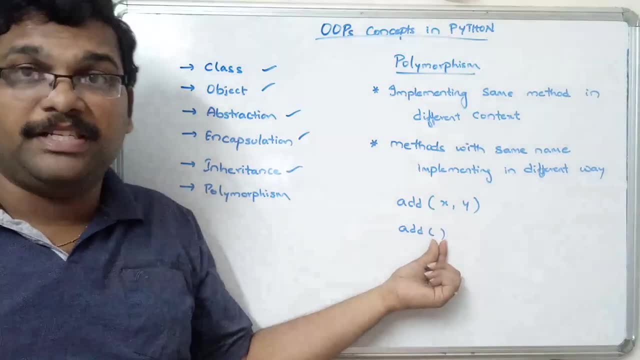 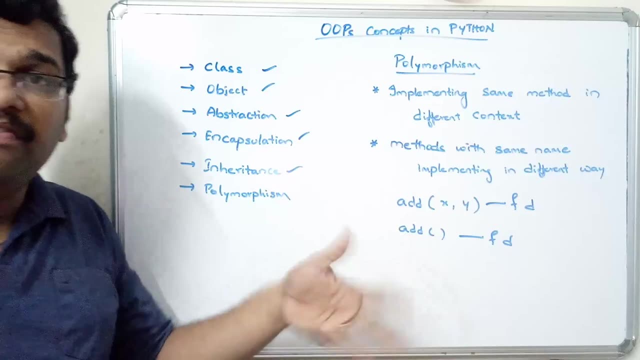 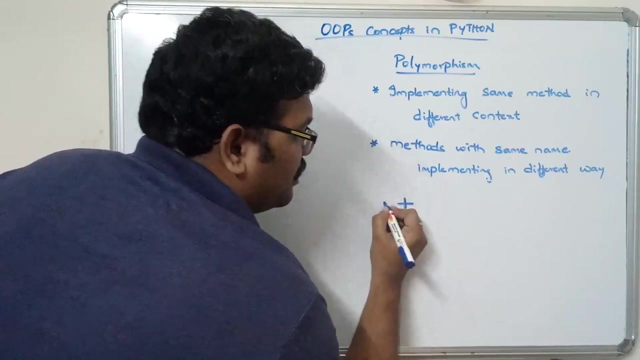 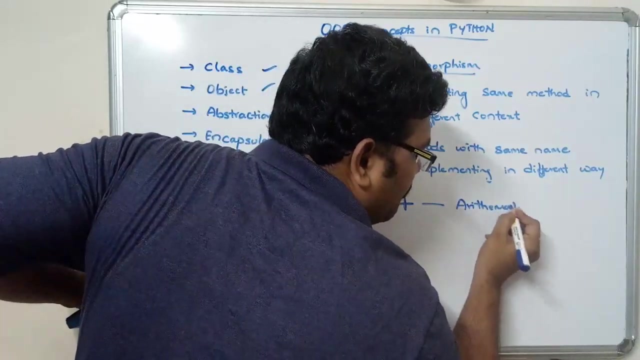 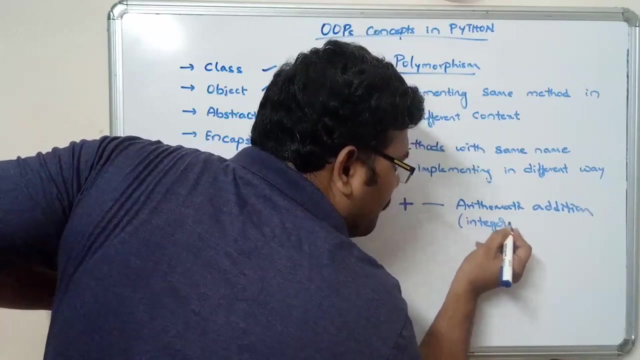 so we are not passing any arguments. so here we are passing arguments, here we are not passing arguments, but this function definition will be different and this function definition will be different, so implementing in different ways. and one more example for better understanding: see plus, consider the plus. so this is the automatic addition for integers and the. 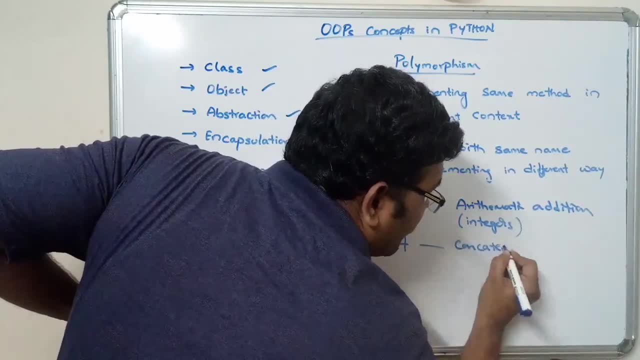 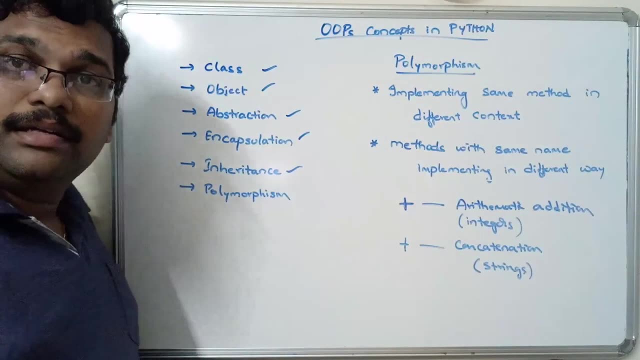 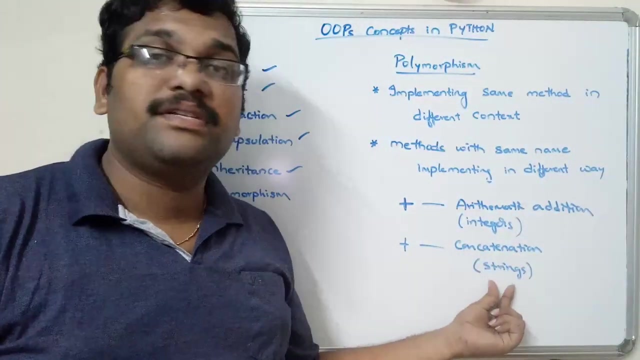 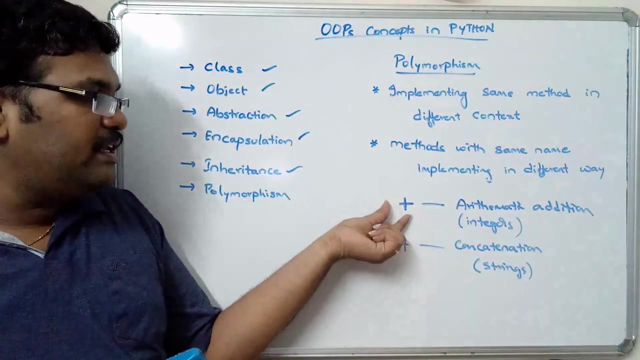 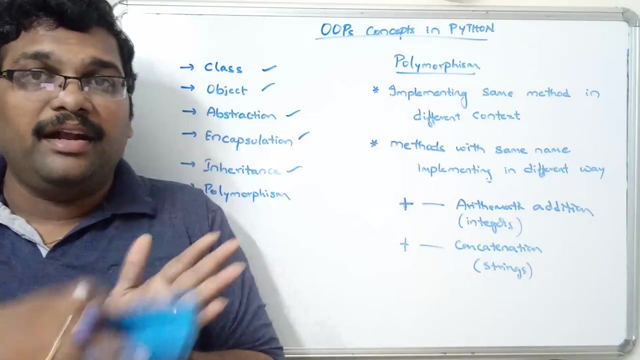 same thing. concatenation in strings, right. so plus is an automatic addition for integers, plus is a concatenation for strings. so same operator implementation is different in different context, so here it is implementing as an automatic addition. there is implementing as a concatenation, so implementing the same method in a different context, in different context. so such type of 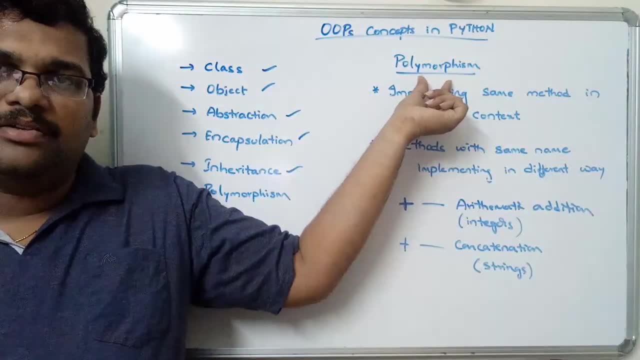 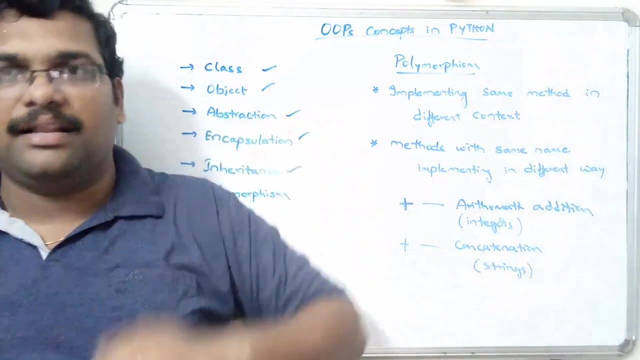 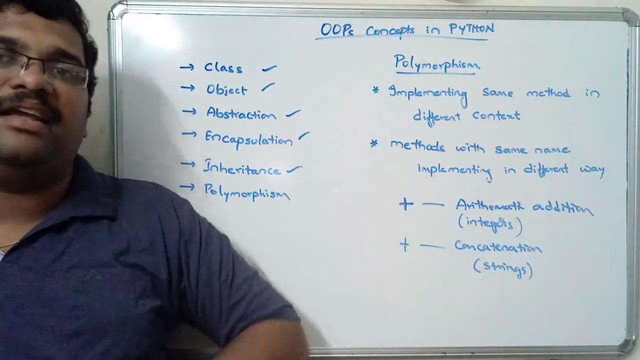 things we call it as a polymorphism. so this completely deals with the methods and inheritance completely deals with the classes. so one class and another class, derived class and a base class, parent class, child class, and here also the polymorphism will be implemented in the inheritance concept. so whereas the